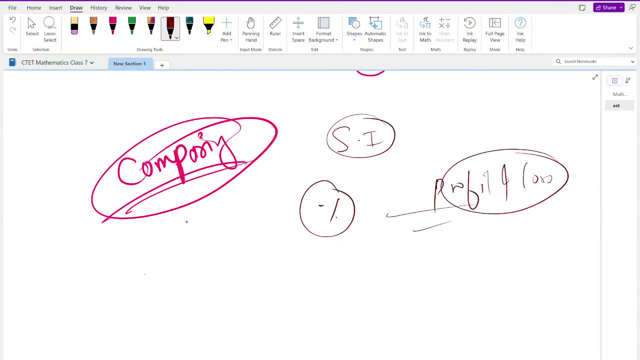 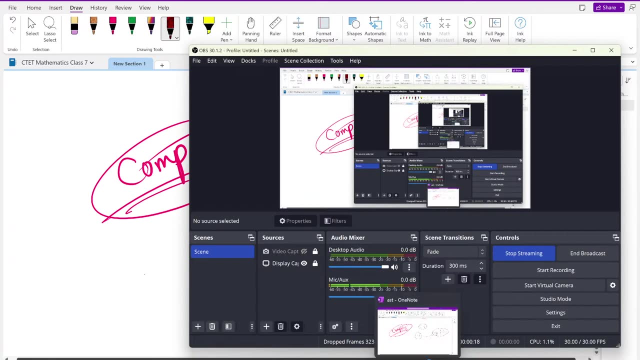 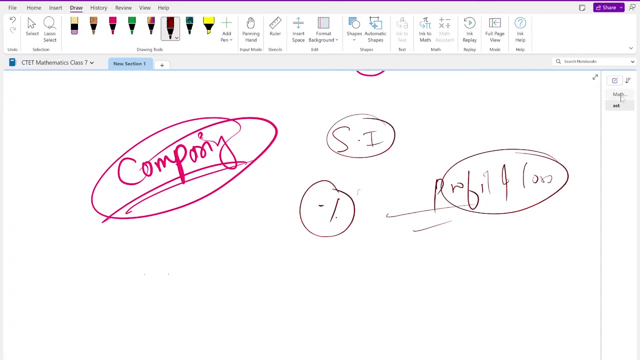 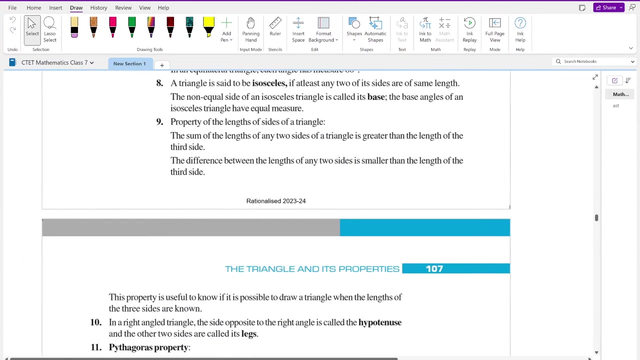 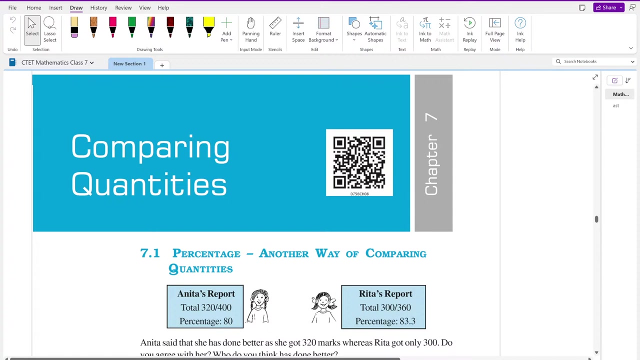 Good evening everyone. Okay, I hope I am audible. Okay, so let's check whether everything is clear or not. Yeah, everything is clear. Chalo. Good evening. good evening, good evening, Hello. I hope I am audible to everyone. 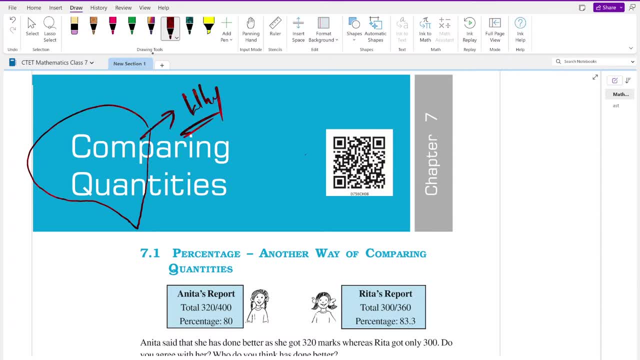 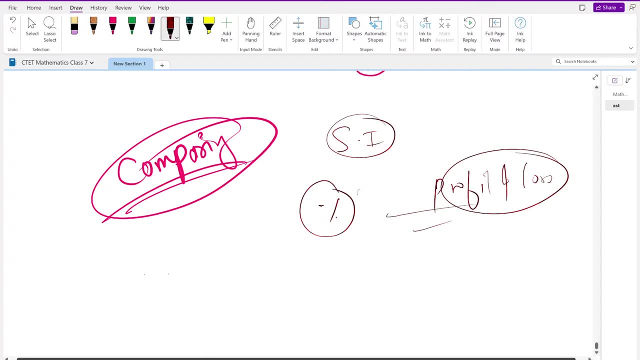 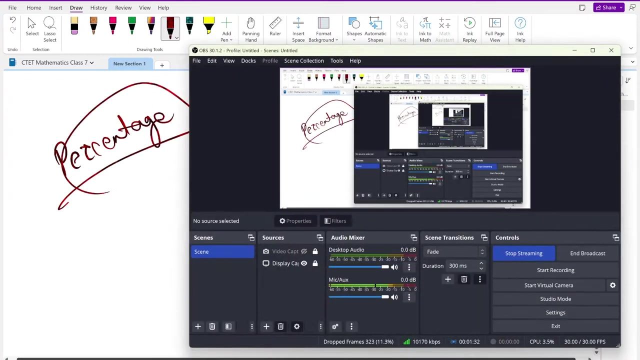 Okay, why? Because here, in this topic, we are going to learn concepts about percentage. Which concepts are we going to learn About percentage? So what and how are we going to talk about this? Okay, percentage. I hope that, as a teacher, you know what percentage is. 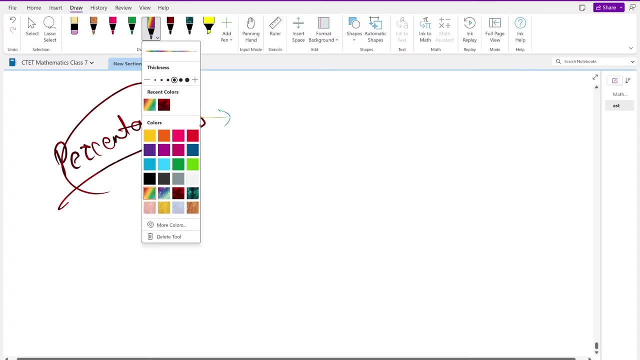 Okay, Okay. and if you don't know, I will explain a little bit and tell you: Percentage means whenever you hear the word percentage, then remember. so how much am I? What am I saying? So how much am I Tell me? this? 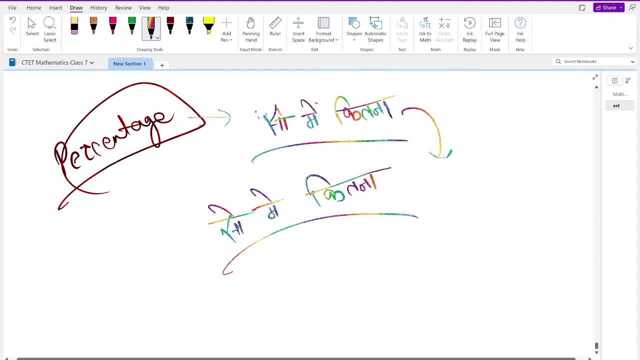 So how much am I? What does it mean? After all, what is this thing? You will get to see different definitions of this, But one simple. what will we call our fatness? Not fat? Okay, Long Basic concept. Okay, This is the right word. What is its basic concept? How much in hundred? Now, what exactly is the concept? How it is. If we get a time and I explain it in detail for the kids, then I will tell you. 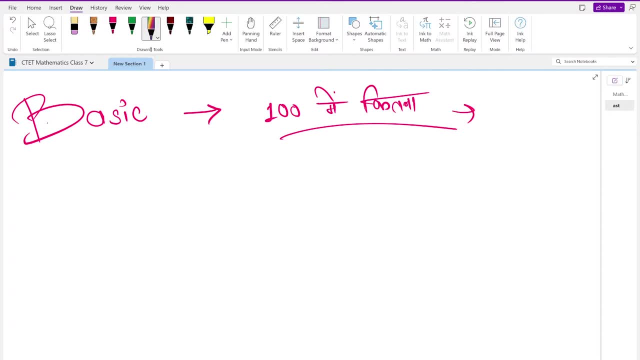 How much in hundre? What does this mean? Look, When we were comparing the quantities. what is it? He is comparing quantities. Let me give you an example. He is comparing quantities. Assume that there is a boy and a girl. 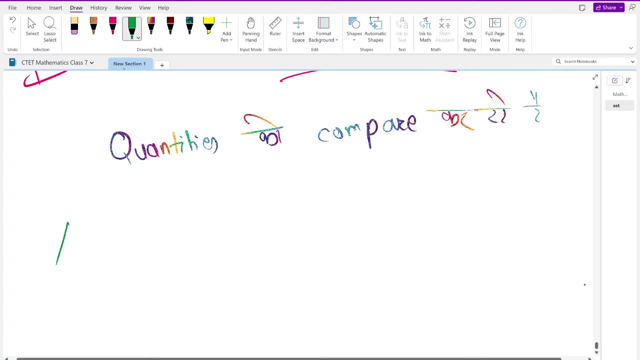 Let's take the girl's name as Ayesha And the boy's name is Sohail. Now understand that there is no difference between names. Now understand a simple thing here: Assume that there is a boy and a girl. Assume that there is a boy and a girl. 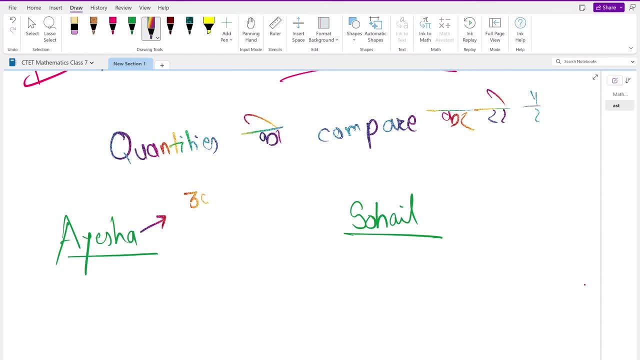 Andских payment are Rs 300. And she spends Rs 90 in food And guest paid Rs 200.. Rs 200 and out of that Rs 100, let's change the value a bit- Rs 150 and out of that Rs 75. 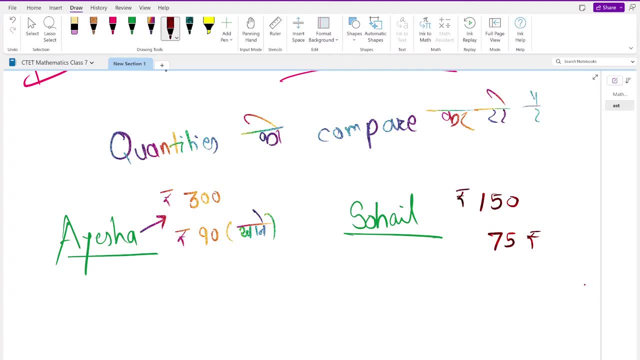 So out of both, according to your payment, who spends more on food? Now, when this question is asked, who spends more on food according to the payment, then here many new students- meaning the child of class 7, will say that 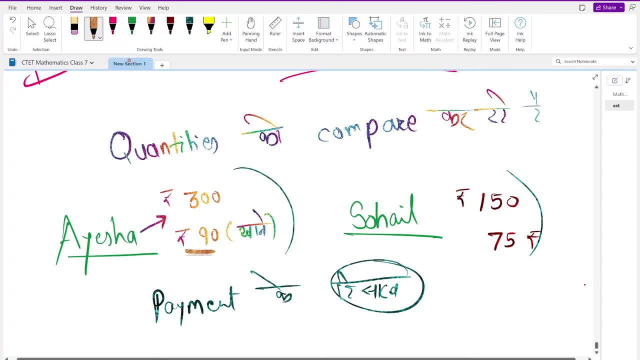 Sir, Ayesha is spending Rs 90 here and Sohail is spending Rs 75, then Ayesha and Dada are spending. So you have to tell there that you don't have to look at just those Rs 90 and Rs 75,. 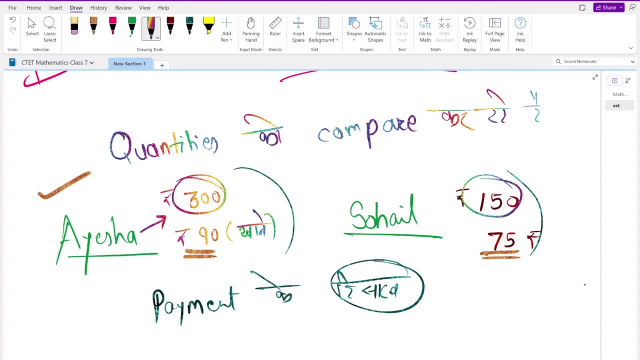 you have to consider the base value of both of them, the payment of both of them, which is Rs 300 and Rs 150.. Are you getting this what I am trying to say to you? Okay, That here, Rs 300 and Rs 150,. 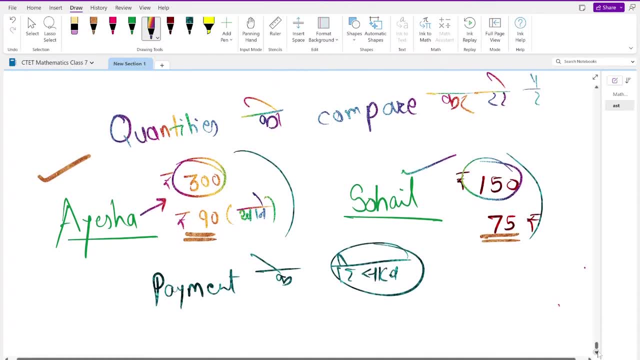 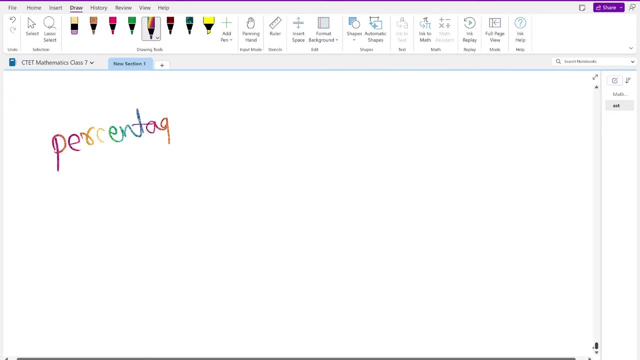 the payment of both of them. we tell: above these payments. then what do we say? We tell here: we will compare them on a common base, Meaning how We will assume that when Ayesha's payment is Rs 300, then she is spending Rs 90.. 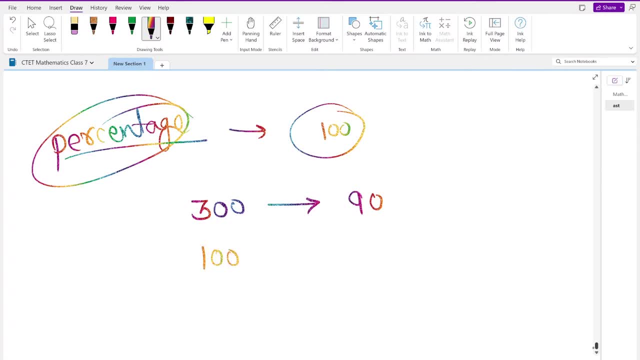 If her payment is Rs 100, then how much will she spend? So we cross-multiply this thing- 90, it has become very thick- 90- into 100 upon 300. And that will be equal to 0 to 0,, 0 to 0, 30.. 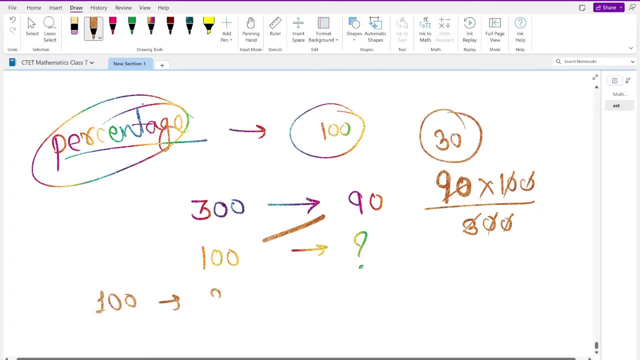 Meaning out of 100, how much money is she spending? Rs 30.. Who? Ms Ayesha? Okay, How much is Ms Ayesha spending? Rs 30.. Come on now let's talk about Sohail. 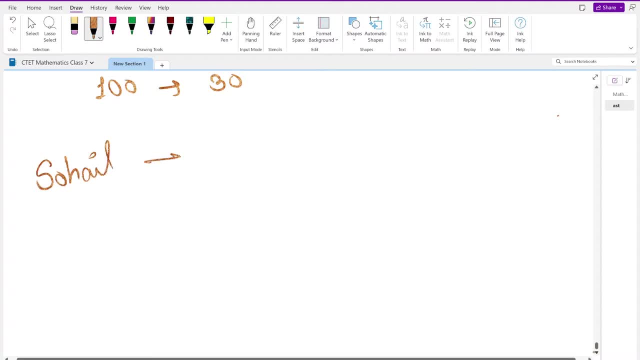 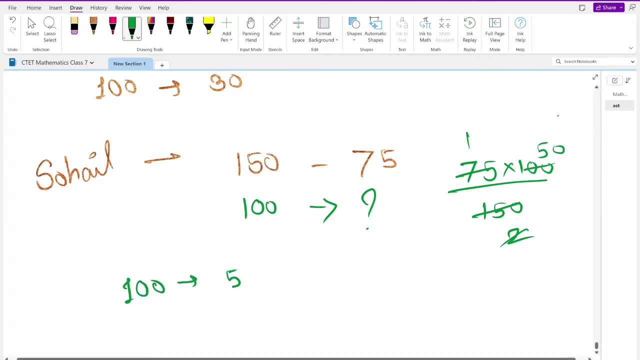 Means, how much money is Sohail spending out of 100? 50, On which we can say that Sohail is spending more money on food? Are you getting this To compare? we took the common thing And what was the common term. 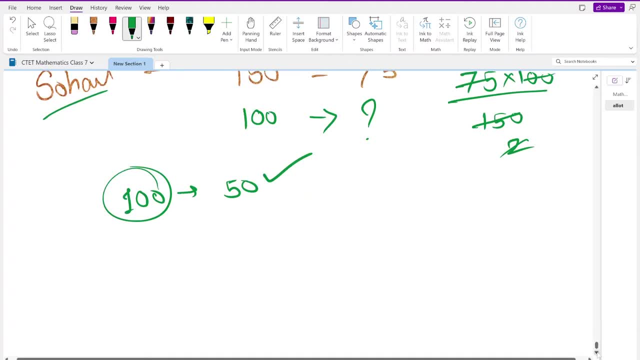 100? What was the common term? 100? Are you getting this Right? So this is what the name of our topic is: Comparing: Quantity. This is because of that. What are we doing? We are comparing On which basis? On the basis of 100. 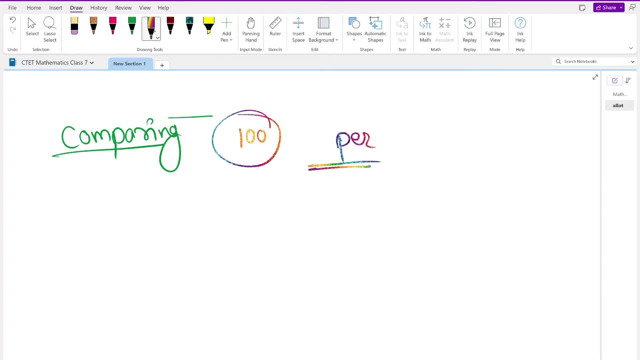 Per means per for everyone, And Cent means 100. So how much in 100?? Tell this means tell the percentage. I hope you got a little bit clear. If we are teaching in the 7th class, So to explain this concept, At least you will get 2 cents. 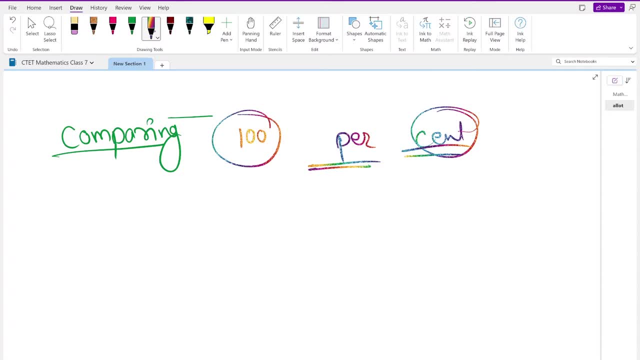 You should give 3 lectures from that. Okay, That is standard time If you ask me, Okay, Come on. Come on. Now we are saying Maybe we will give some examples, Some definitions. We will talk about those examples and definitions. See Now. see, There is a definition in the book. 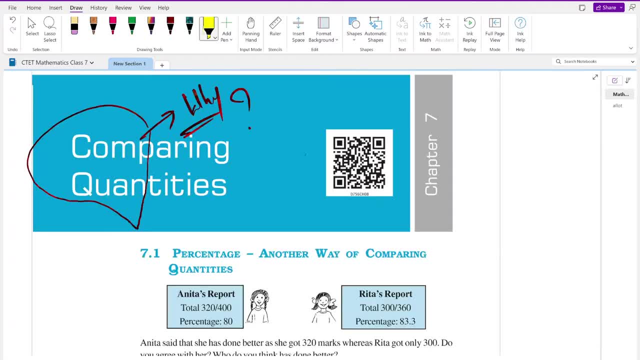 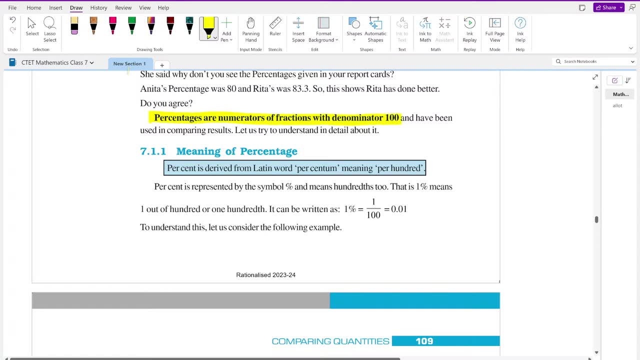 What is the definition? Let me show you Percentage. Are numerators of the fractions With the denominator 100? Any fraction When the denominator is 100, So the numerator of it Tell the percentage Means. I wrote 75 upon 100, So read it: 75%. 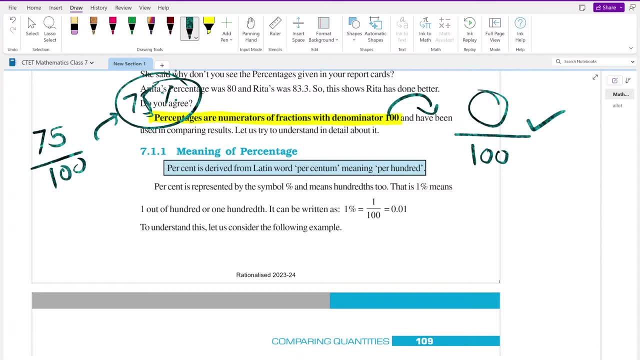 Read it: 75% Means Indirectly Here. Remember this: That Percentage sign Whenever you see it somewhere. It means 1 upon 100. What does it mean 1 upon 100? Does everyone understand this? What does percentage word mean? 1 upon 100? 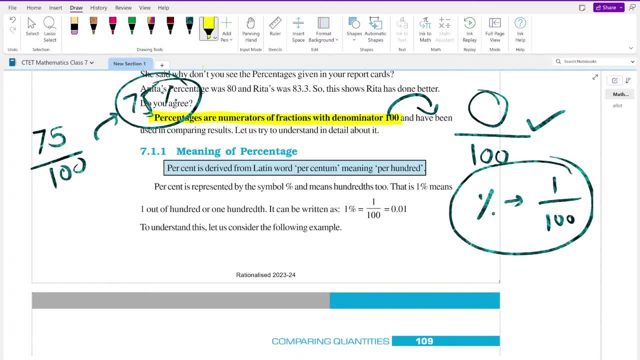 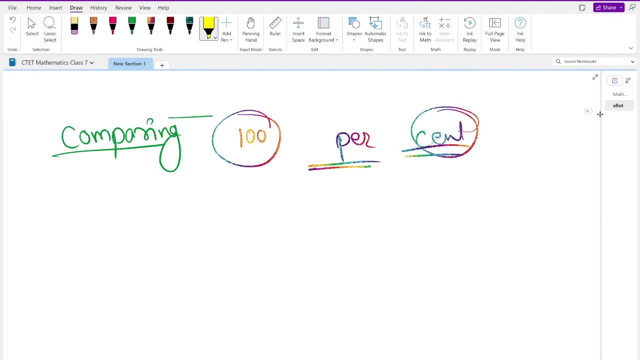 Is it clear to everyone? Okay, Percentage is a term, Latin word: Percentum Means Per 100. It is taken from above. Okay, This knowledge is also important for us. Now come forward. See Fraction And percentage. There is a relation, And what is that relation? I would like to tell you. 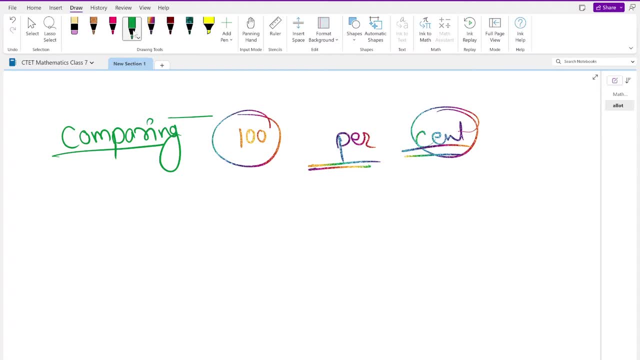 Assume, Say any name. Okay, Let's take Ayesha's name. Okay, Ayesha is, She has 100 bangles. She has 100 Bangles Which? Yellow, Green, Red And Blue And Blue. Okay, Now understand. I said They have 14 bangles Yellow. They have. 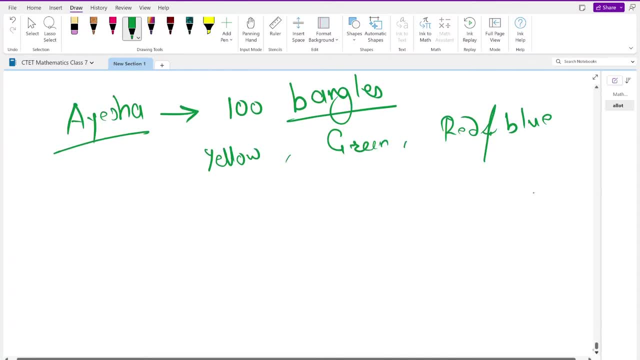 14 Bangles Yellow, 26 Bangles Green. So They have 14 Bangles Yellow, 26 Bangles Green, So They have 35 Bangles Red And 25 Bangles Blue. So Tell me, Can you tell me Its Fraction That? How many yellows are there in the total? 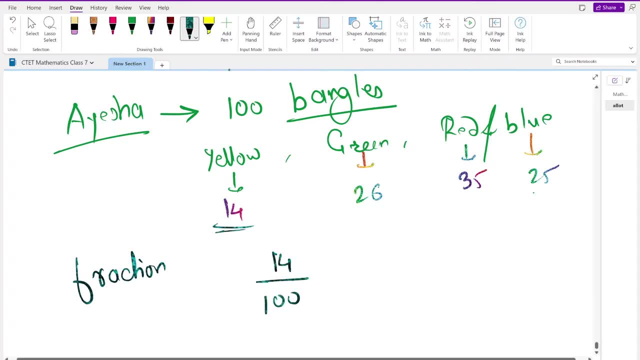 Absolutely 14 upon 100. We know We take the total value in the denominator And from that selected value We take in the numerator Right. See here 26 upon 100, Here 35 upon 100, Here 25 upon 100. Now, What did I tell you just now? 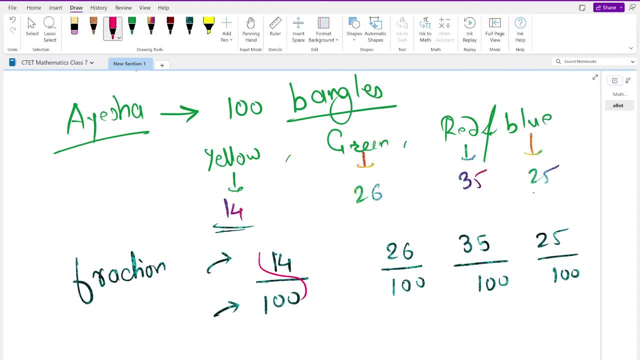 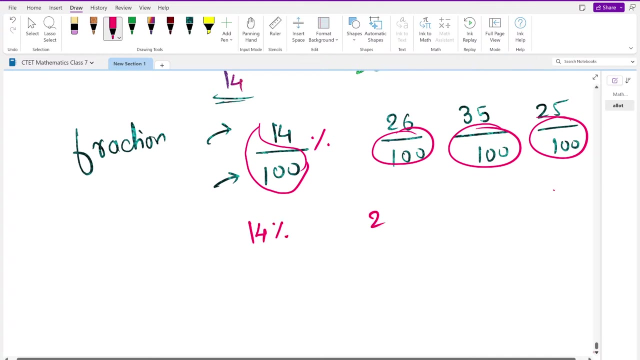 What did I teach you just now? That this 1 upon 100, This 1 upon 100, We can Change it From Percentage. This Is 14%, This Is 26%, This Is 35%, This Is 25%. So Got it, Got it. 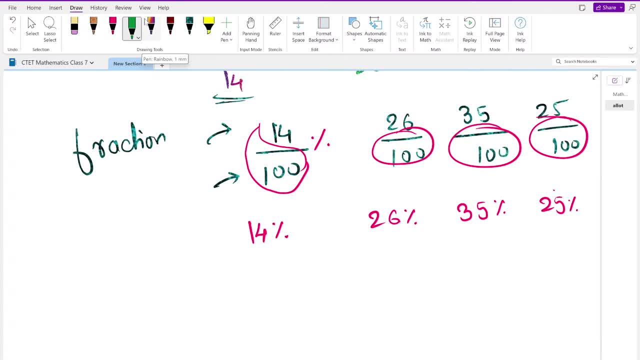 Fraction And What is the relation of percentage? If you Fraction Upon 100, Denominator 100, What do you do if you Denominator 100, So that fraction We will Call Percentage? What will we call that fraction? Percentage Means, Can I About Ayesha? Can I say? 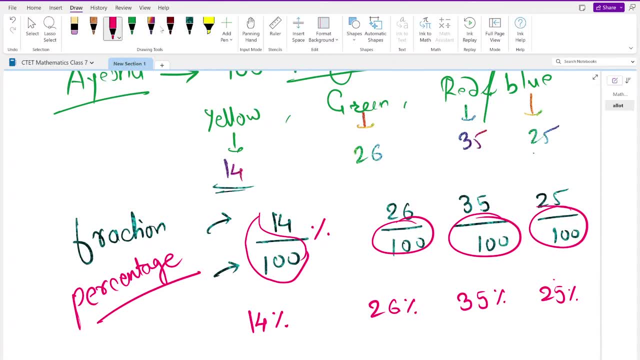 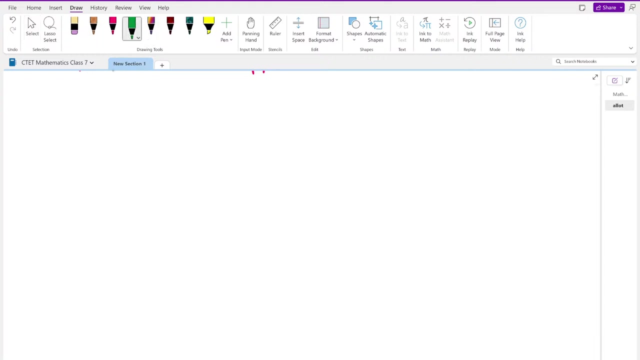 That Ayesha Has 14%. How much? 14% Is Yellow, 26% Is Green, 35% Is Red And 25% Is Blue. Does This? Everyone Understand This? Good, Now, Understand A Thing. I Here, I Thought Not at all, But they are teaching this to the students in the 7th class. 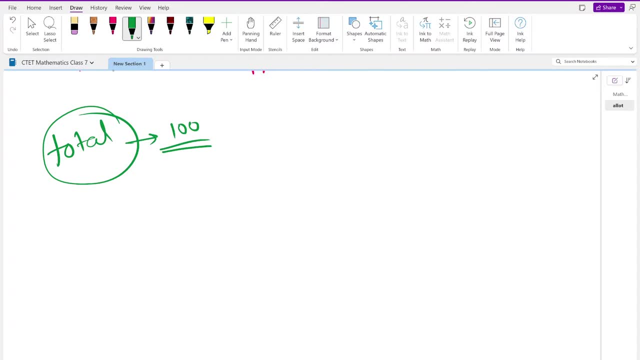 That's why they didn't tell you in the beginning. So let's assume they solved the total of 100. But that won't be always the case. Okay, Always remember this. Now I will teach you how to solve the problem when there is no total of 100. 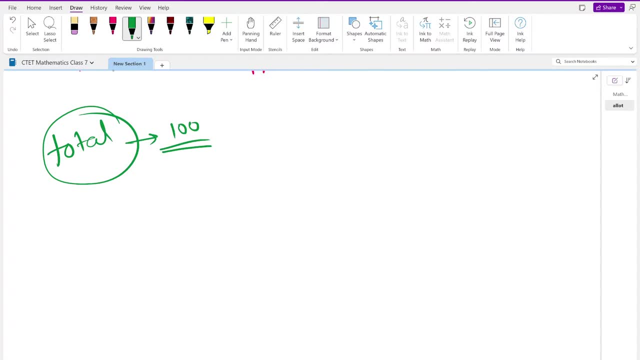 Let's assume a person has. Let's take a name, Let's take my name. Which one is bad? Okay, Pay attention, Is it Abdul? Abdul has red and blue. Okay, He has 10 marbles. Red and blue are equal. 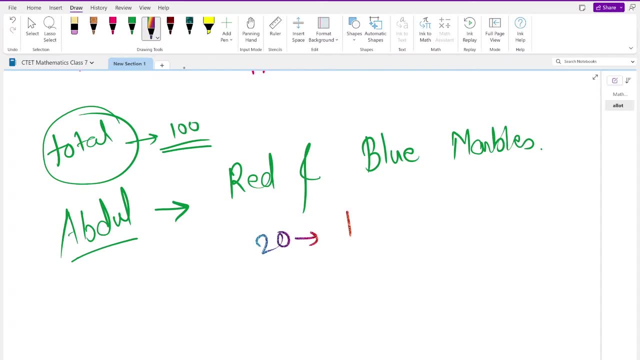 He has a total of 20 marbles. He has a total of 20 marbles, Of which red is 8 and blue is 12.. So how will you tell in fractions How many red marbles does Abdul have? 8 by 20.. 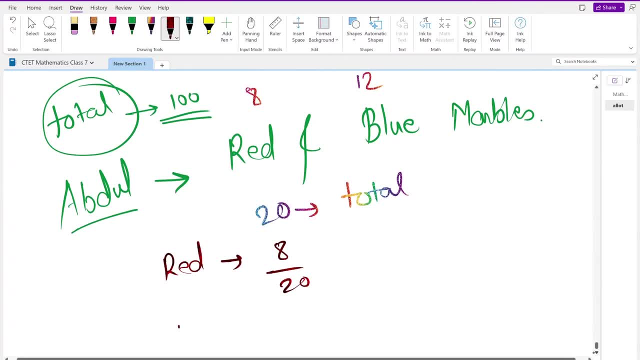 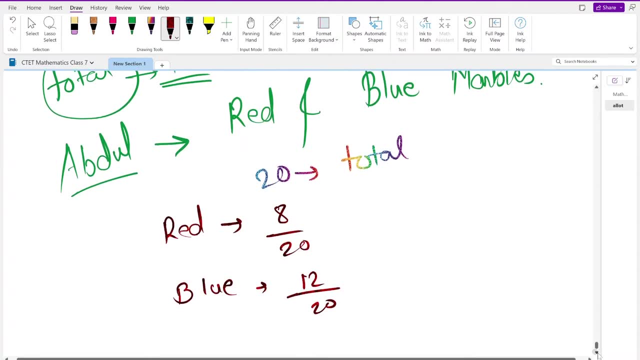 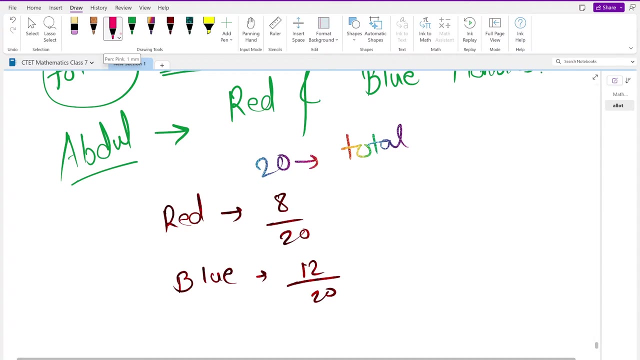 How many blue marbles does he have? 12 by 20.. So I told you that if you want to tell a fraction in percentage, then make the denominator 100.. How can we make it 100? Two options. Multiply it with 100 by 100.. 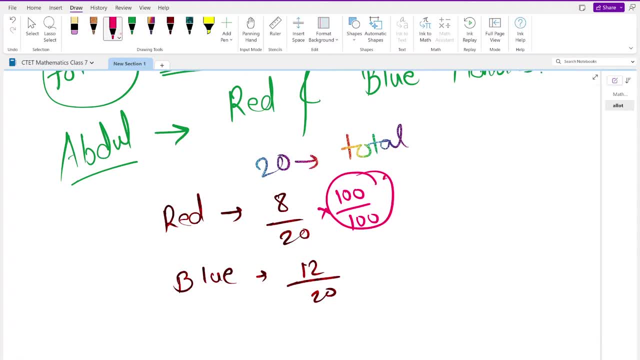 Why? What is the meaning of 100 by 100?? It is 1.. And if you multiply any number with 1, then there is no difference. That's why I am saying: multiply it with 100 by 100.. Or, if you are smart, 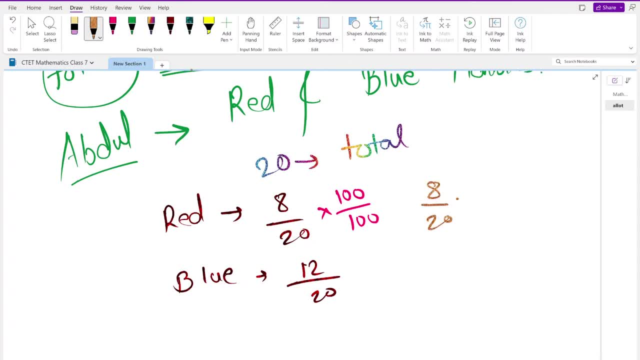 then you can see here 8 by 20. If we multiply it with 5 by 5.. So 20 times 5 is 100. And 8 by 5 is 40. So 40 by 100. And this is 40%. 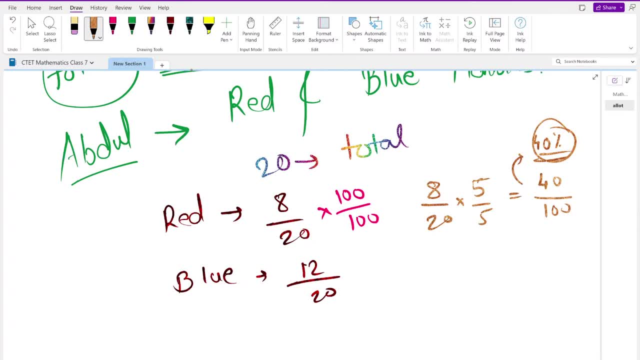 If you can see this, What is it? 20 into 5.. If it is 100.. If you remember this well at that time, at that time, then you can do 40% easily. And here also the same Into 5 upon. 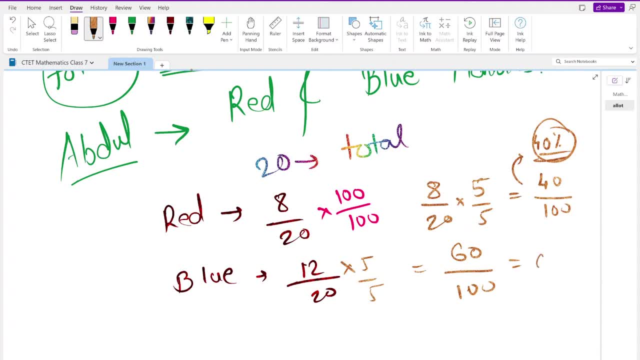 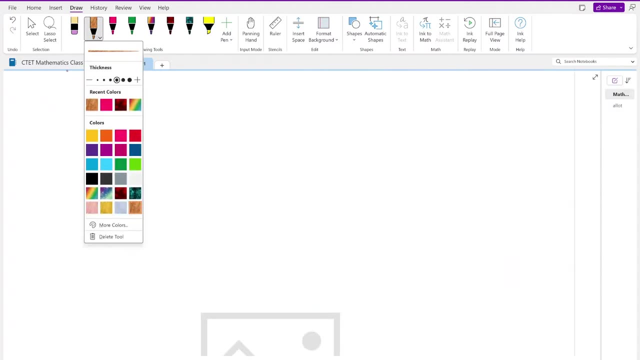 5. That will be equal to 60 upon 100. And ultimately, 60%. Did everyone understand this thing for sure? Okay, Come on. There are some more examples in the book. Let's solve those examples. Okay, Come on. 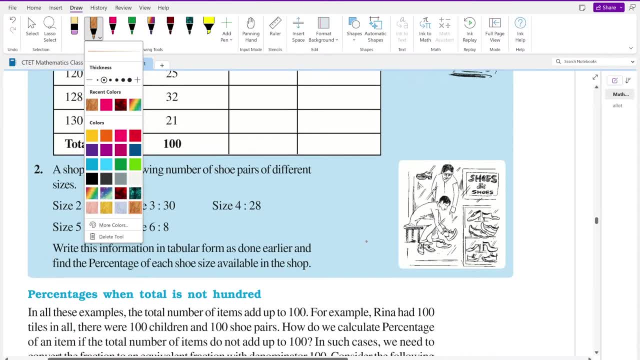 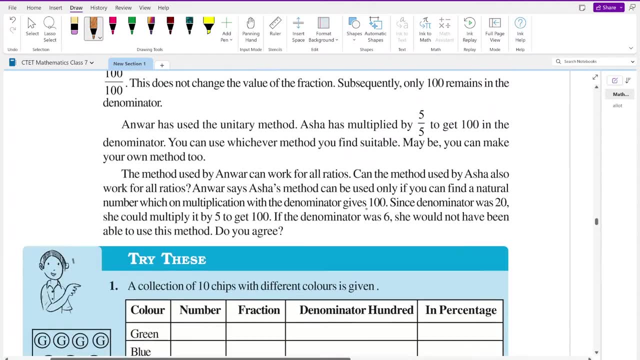 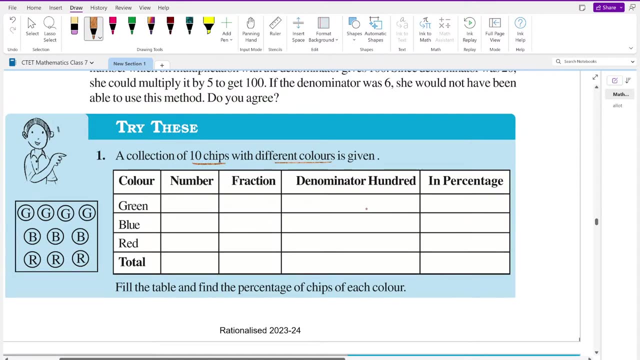 Get ready Now see Green: A collection of 10 chips with different colors. Okay, See How much is green: 1, 2,, 3, 4.. How much is blue: 1, 2,, 3.. 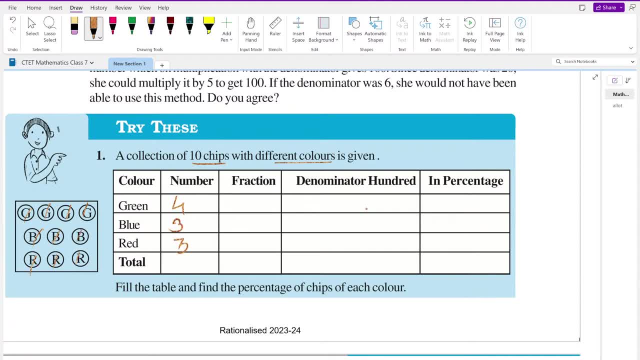 How much is red? 1, 2, 3.. How much is total? 4 and 3.. 7 and 3.. 10. Say fraction 4 by 10.. Say blue: 3 by 10.. 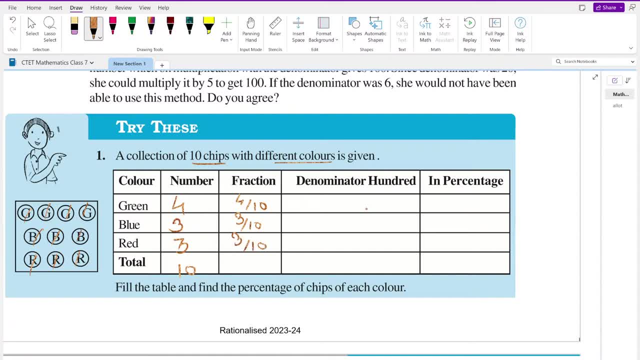 Say red: 3 by 10.. Total 10 by 10 means: 1. Convert this into 100 denominator. Now you understand this right. 4 by 10.. What am I saying? Pay attention. 4 by 10.. 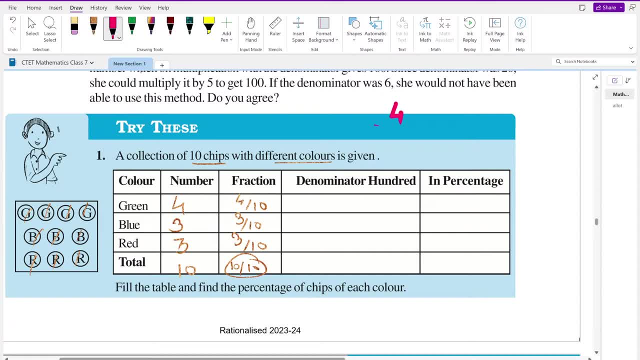 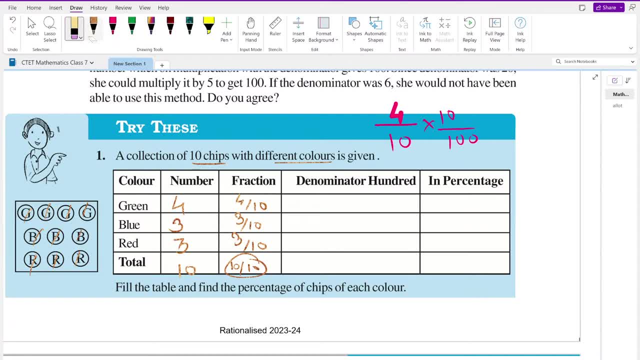 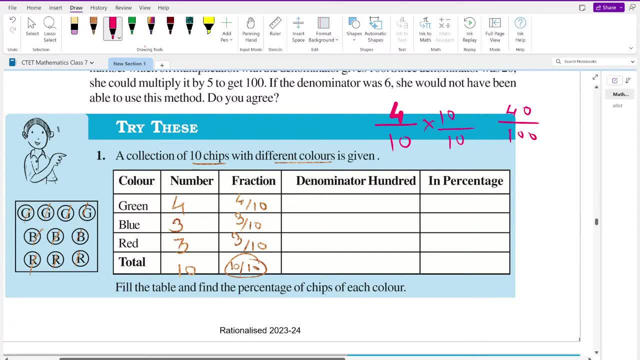 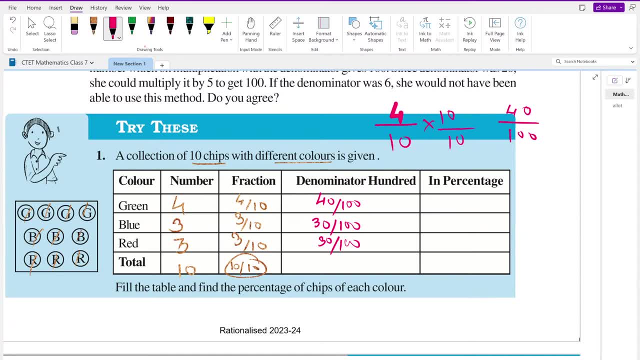 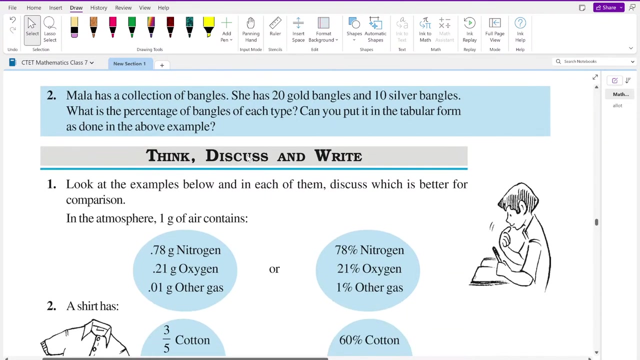 10 by 10.. 10 by 10.. I hope every one would understand this. I hope now you gave perfect answer to this problem. hmm, what is the next question? mala has collection of bangles malakipas. bangles ka collection hai, 20 gold ke 10 silver ke hai. 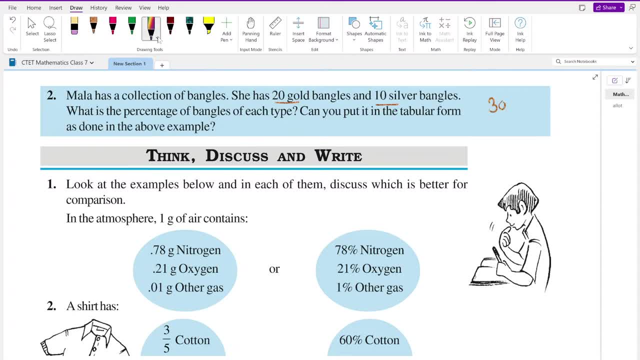 total 30 hai. what is the percentage of bangles of each type? sabse phale hum kya karenge? gold ke nikaalinge, okay, gold ke nikaalinge, 20 upon 30 into 100 by 100 sahi hai, okay, nikaalo zero, zero, cancel. 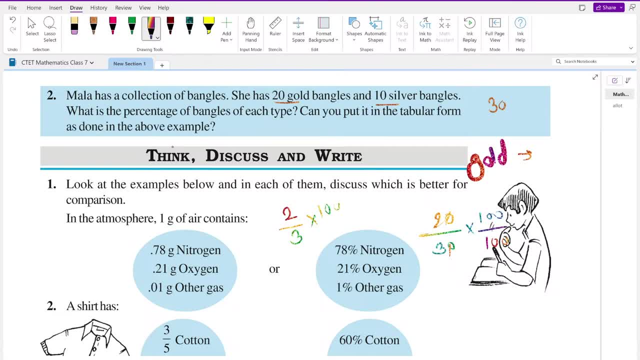 two by three into hundred by hundred. ab dekho, yeh upon hundred hai. isse hum sida percentage. lele kunsa yeh upon ka hundred. to yeh kya hoga? 200 by 3 percentage, maine, kya kya yeh baat pakka har kisi ko sumaj mai. 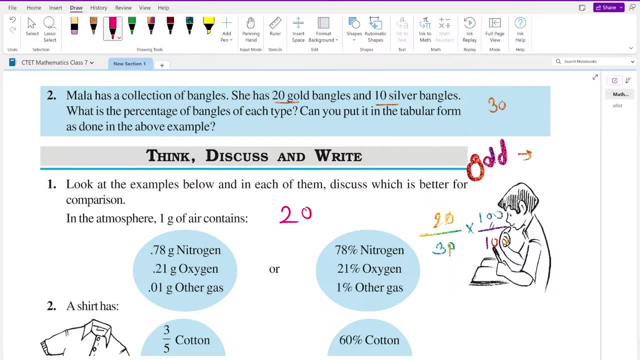 mai yaar par tumhe firse likh kar batata hu: okay, dhyan dega har koi two upon three into hundred by hundred, aur yeh jo upon mein hundred hai. uske liye mein seda percentage ka symbol le rahe hum. 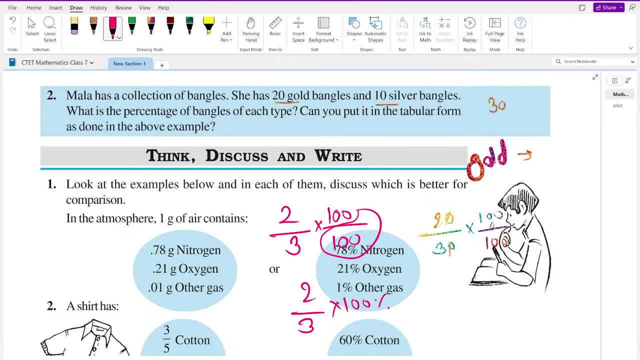 two by three into hundred percentage. aur issi ko mai aage likh sakta hu, 200 upon 3 percentage. ab karo se solve 3600, 18, 3600, 18.66, wo kab tak bhi aage chalega? recurring kate usse. 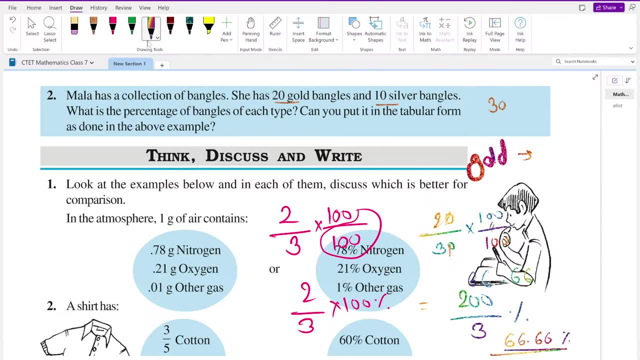 to phir yeh percentage ho gaya 66.66. i hope yeh baat pakka. har kisi ko sumaj mai aai hoge gold ka kitne percentage bangles hai, maala ke paas 60.66, 60.66. 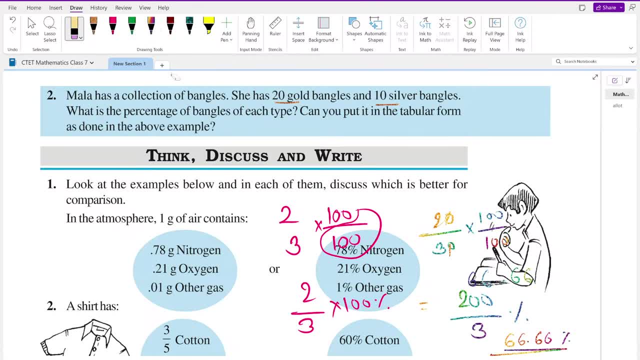 right, ok, chalo gold ke baad aate hap silver ke pay, silver ke kitne bangles hai maala ji ke paas. ten, yes, okay, likha usse. ten by 30 into hundred, by 30 per cent. What will I write? 10 by 30 into 100%. 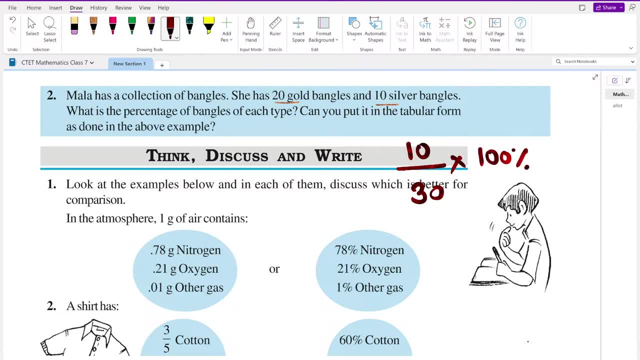 Now, how can I write 100% directly? What does it mean? How can I write 100% here? Because I know that I have written 10 by 30 into 100 upon 100.. And what term did I use for upon 100?? Percentage. 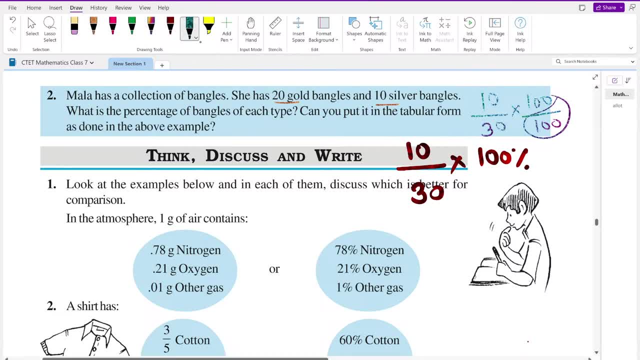 I hope this is clear to someone. Let's solve it. 10 by 30 means 1 by 3 into 100%, So 100 upon 3% means 33.33%. Is it easy? Very good, So how many gold bangles does Mala Ji have? 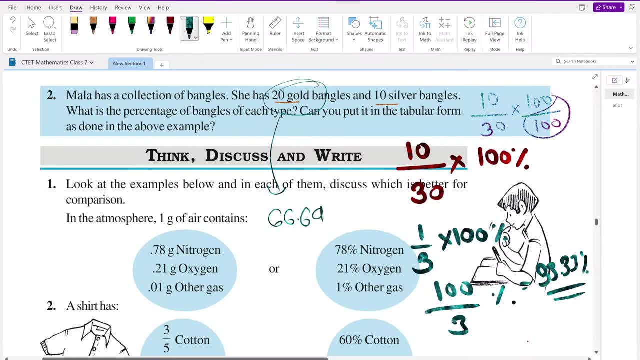 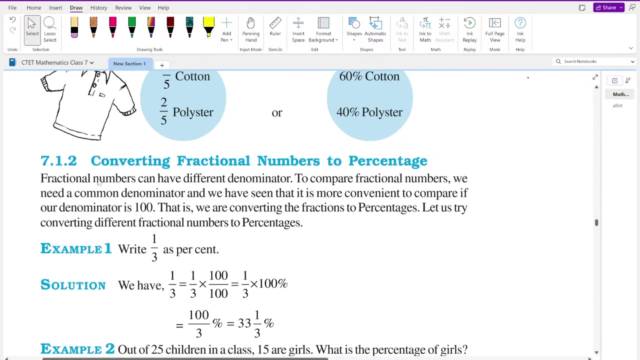 66 points. Okay. 66% and 33.33% of silver- Okay, I hope this is clear to everyone. Okay, Let's go Now look, Pay attention. There will be some questions on this. Let's solve these questions. 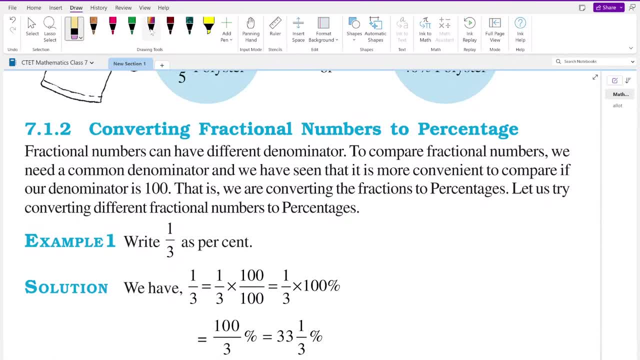 Okay, Write 1 by 3 as percent. What does it mean? Write 1 by 3 as a percent. So how will we write? It's simple: We have to write 100 upon 100. Then we will convert this upon 100 into percentage symbol. 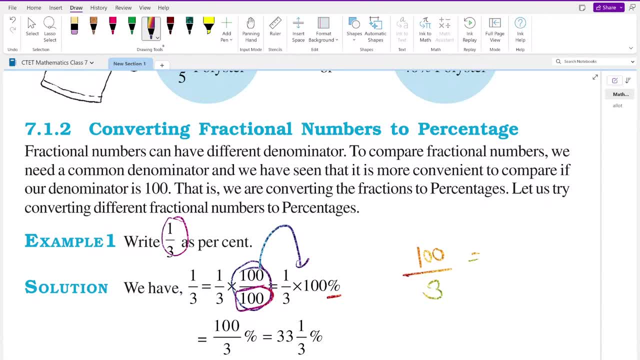 Then we will do multiplication 100 by 3.. We know that we can convert improper fraction into mixed fraction. Absolutely How, 33.. 1 by 3. Percent. How to do this? Please don't ask this question. 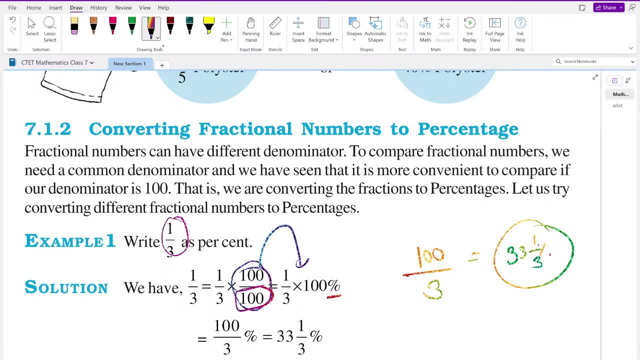 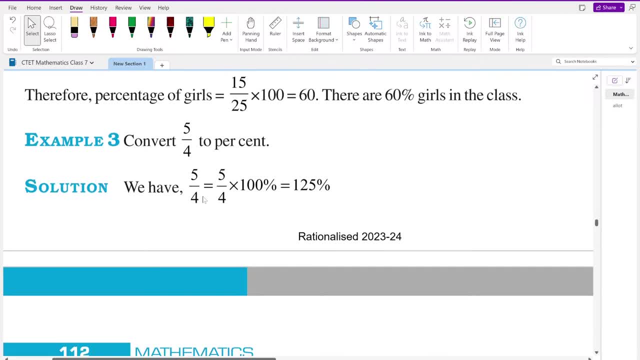 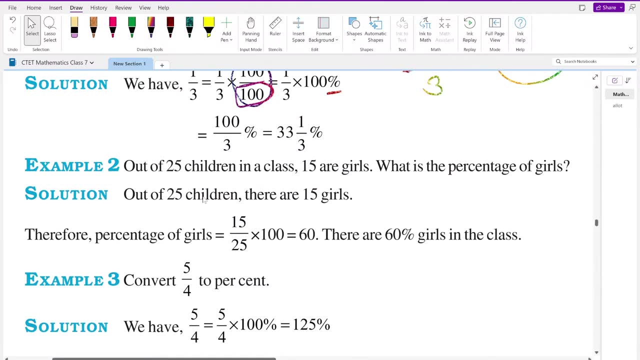 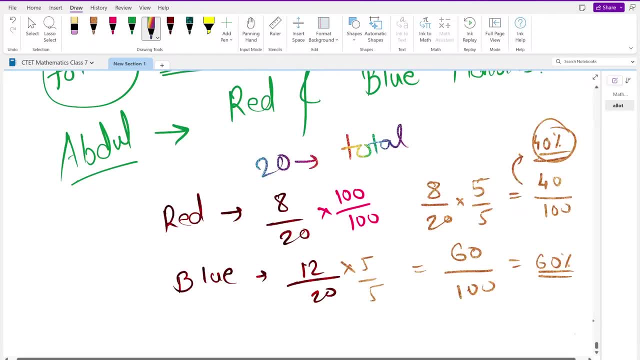 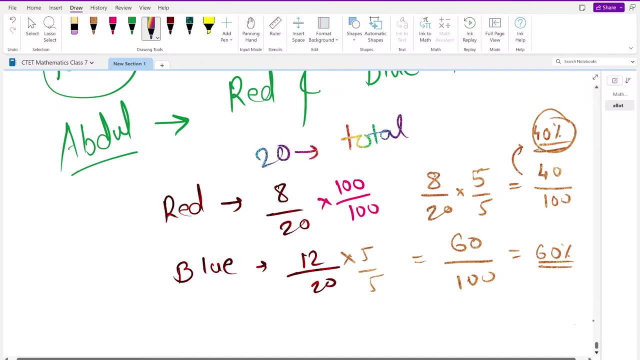 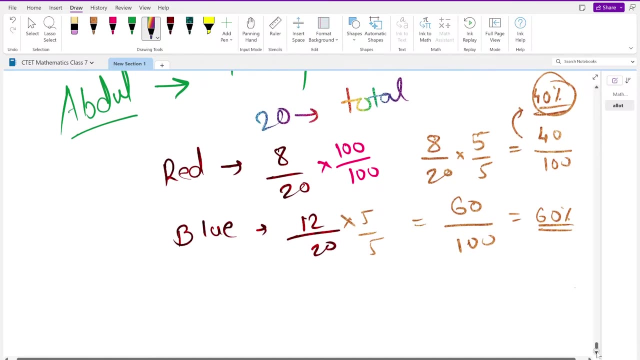 Okay, Alright, I will solve this question. I will answer two questions for you. Hmm, I think what was the question? 25 students, 23 from 25 students, Right right from that, 15 or 10, 15 girls, 10. 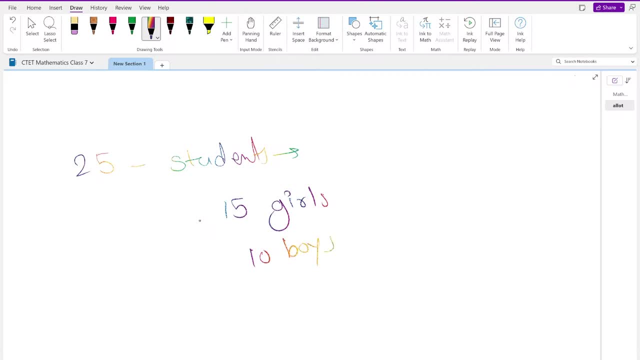 boys. ok, first of all i will ask you a question: tell the percentage of girls and boys. ok, first take it in fraction: from 15 girls, 25 boys into 100%. now see, solve it. everyone knows table of 5: 25 x 1 is 25. 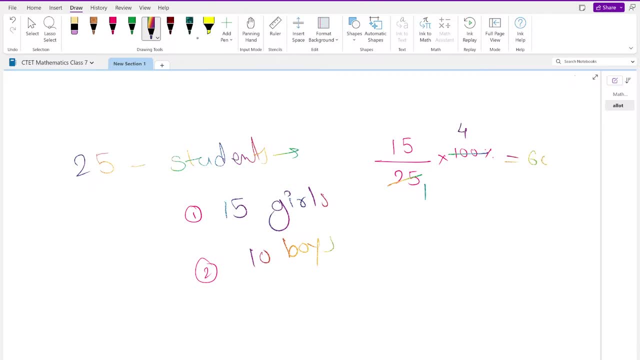 25 x 4 is 100 and 15 x 4 is 60. so who is 60% girls? 10: 25 x 2 is 100, 25 x 4 is 100 and 10 x 4 is 40. 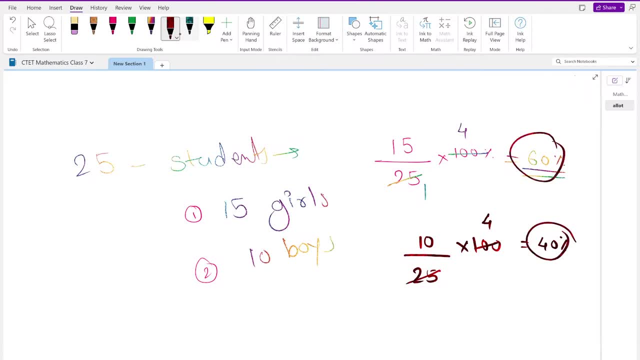 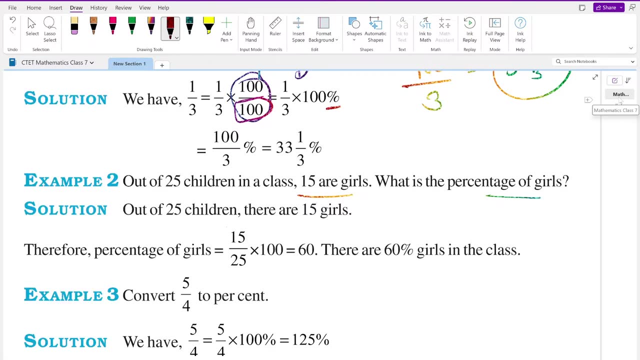 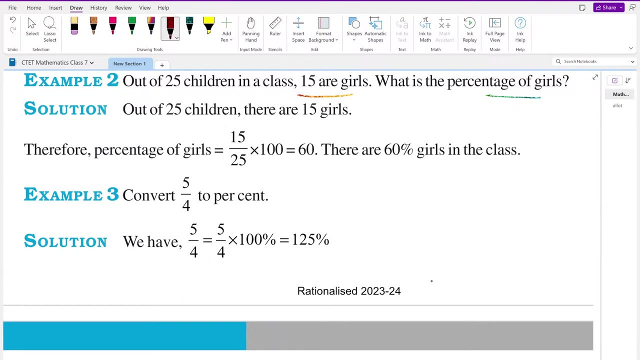 so 40% boys from fraction how you have to get percentage. i hope everyone understood this is not difficult, but practice is necessary. this comes in many competitive exams. convert 5 x 4 to percent. what is said 5 x 4 to percent. convert it to 100%. 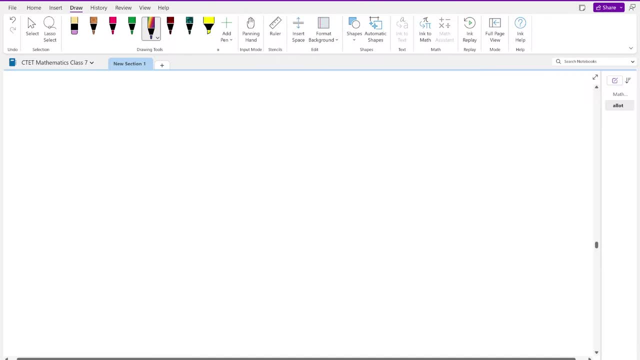 hmmmm, hmmmm, hmmmm, hmmmm. now see, when you see 5 x 4. ok, when we see 5 x 4, 1 minute. when we see 5 x 4, we can make it into 100%. this is the one way. 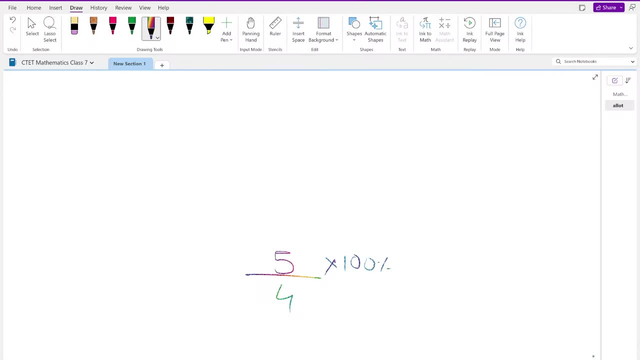 what is one way? Just a minute, Just give me a minute. We can do this: 5 by 4 into 100%, Or 5 by 4 into 25 upon 25. Why? Because if we do 25 into 4, The denominator will be 100. 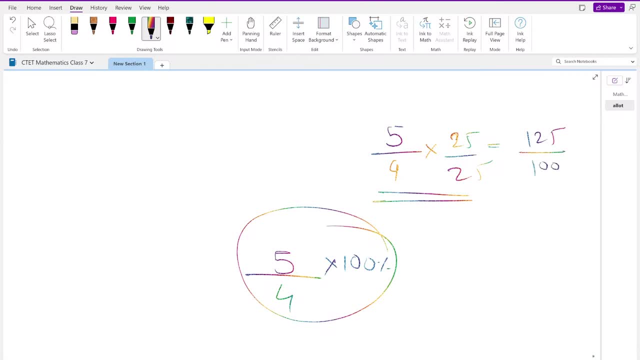 25 by 5 is 125 And this is 100, And this 100 Take the percentage 125%. Is this clear to anyone? Clear? Okay, let's go Now let's come to the next question. What is the next question? Is the next question here? 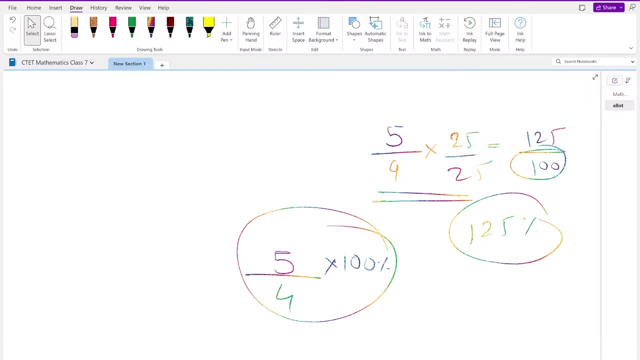 Wow, there are a lot of parts in this. Okay, in this lecture We will just do the theory part. We will solve the exercise and questions in the next lecture. It's not a big deal. Now see The next part. we have to learn. We have to convert the decimal into fractions. 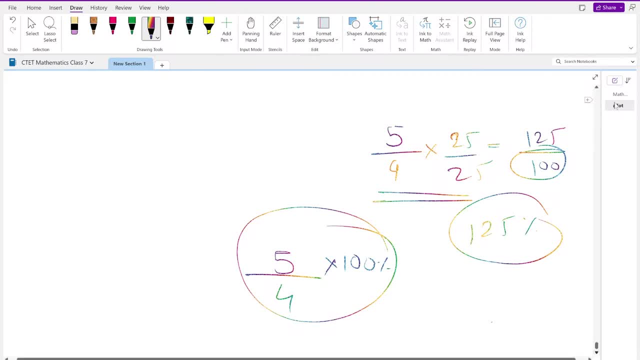 So what is that? Let me show you. Oh man, I don't know why this channel gets less and less in its life. Now see, I gave you any number, I gave you 0.75 And I told you to convert it into percentage Straight. Multiply it by 100. 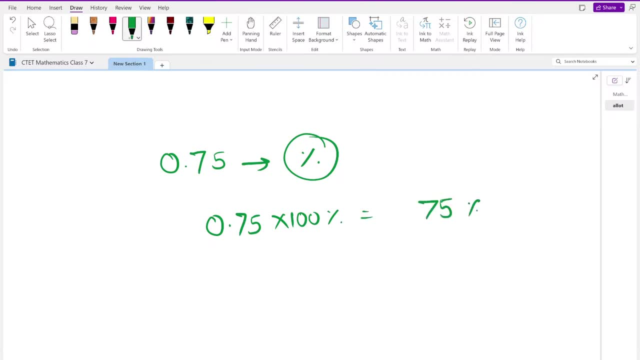 And put the percentage symbol. So this is 75%. Is it that easy? Is it that easy? Yes, life is so easy. I wrote 0.2 into percentage, 0.2 into 100%, And that is equal to 20%. 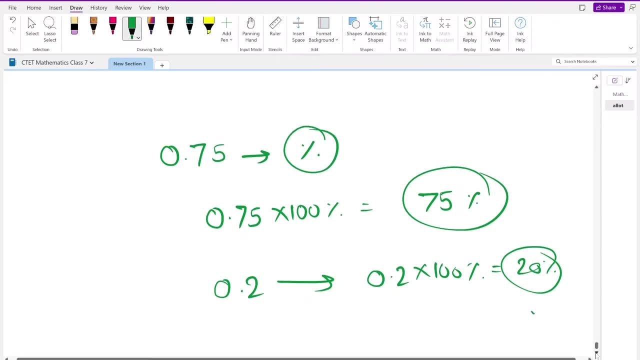 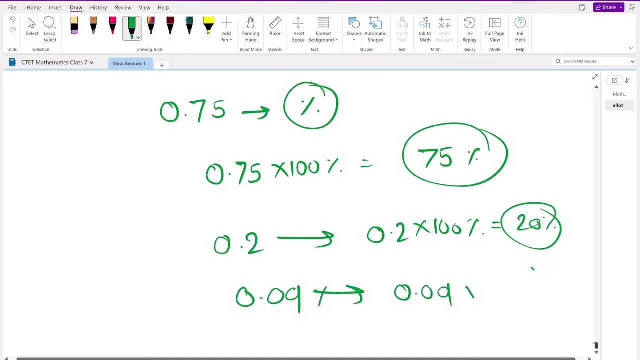 Is life so easy? Yes, it is. This is normal life And mental life is the same. I wrote 0.09%. Sorry, 0.09. So what? 0.09? Multiply it by 100 And put the percentage symbol 0.09 into 100. 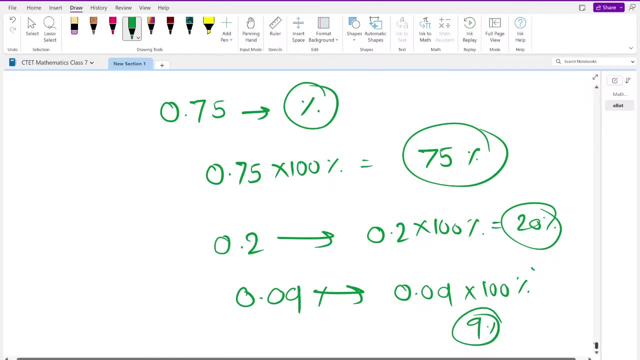 9% Done. Yes, this much is easy. Now see, We have some questions. Let's talk about those questions. We have been told To convert 12 upon 16 into percentage. So first of all, I simplified this 3 by 4. How? How? 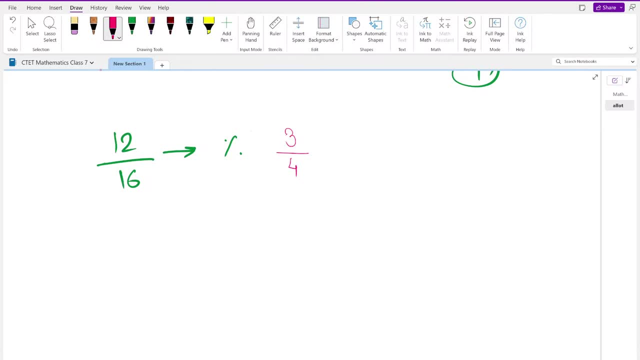 I know the table of 4. In the table of 4, 4, 3 is equal to 12, 4, 4 is equal to 16. So then it is done. And now I multiply it by 25 into 25, So this is 75 into. 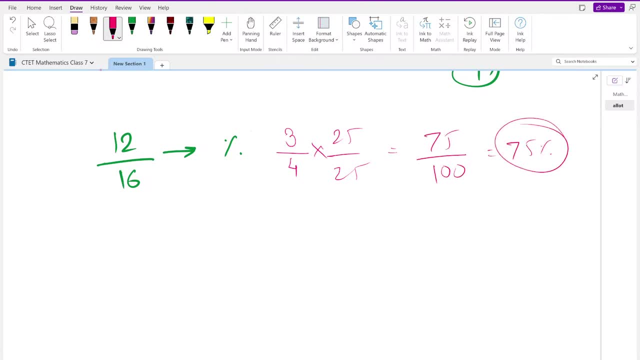 Upon 100 And that will be equal to 75%. Done, Easy peasy, Sure, sure, sure Good. Come ahead Now. we have been told: 3.5 into percentage. Convert it into percentage. It is simple: 3.5 into 100%. So this is done. 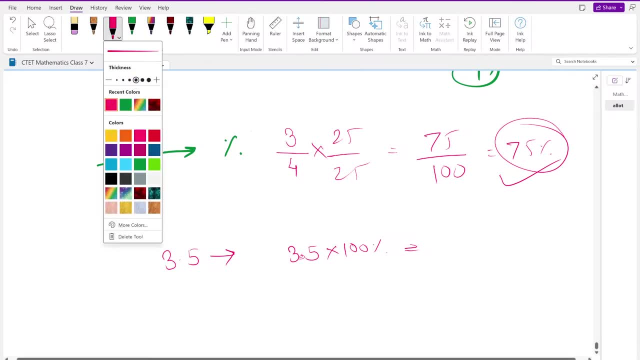 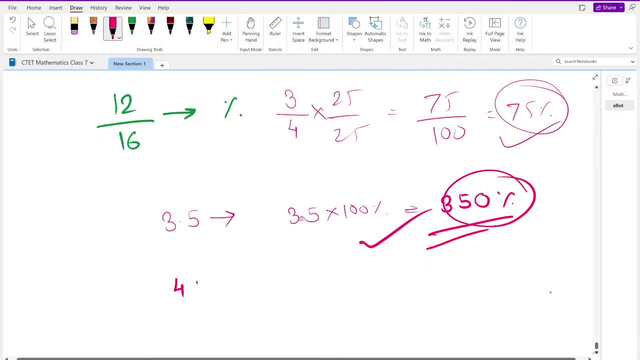 Let me make it a little bigger in life: 350, 350%, Right, Okay, let's go next. Now see, Now it is said 49 upon 50. Convert it into percent. I, just I am doing 2 upon 2, It will be 98 upon 100. 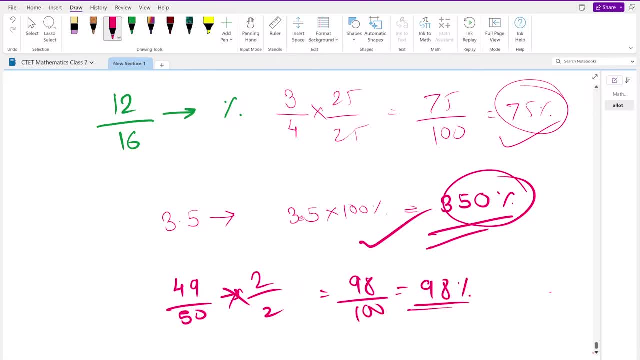 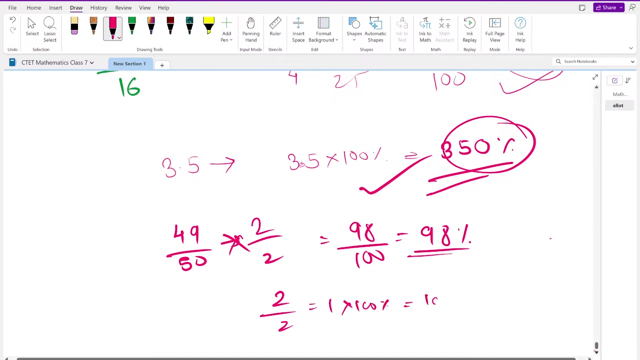 Which is 98%. Are you sure you understand this? Okay, Look at the next question. What is the next question? In the next question it is said 2 upon 2. 2 upon 2 means 1, 1 into 100%, 100%. 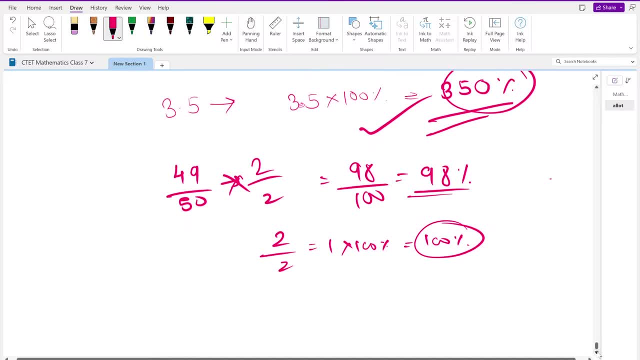 Done. Now see, 0.05 is said Into 100%. So it is here: 5%. Easy, Yes, Very easy. Okay, Come on, Let's talk about the next question. What is the next question? It is said in the book, And I hope everyone has a book. 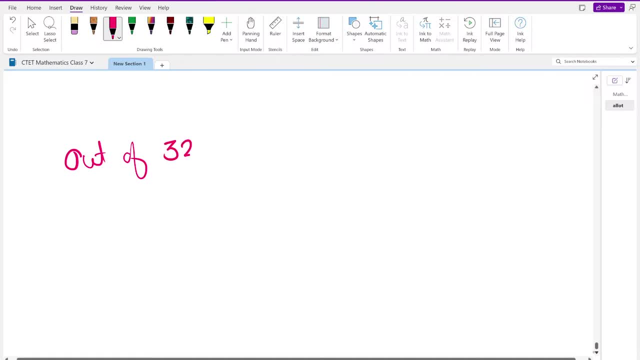 Out of 32 students. Out of 32 students, 8 are absent. 8 are absent. So the percentage of absent students, It is said to tell How will we get it out? First, take the fraction: 8 are absent From 32. So this is done 1 by. 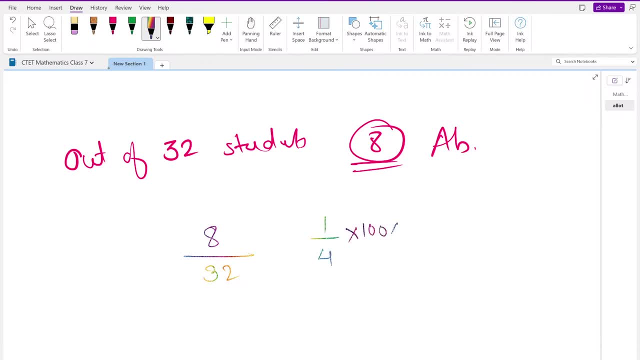 4 Convert into percentage, So into 100%, And this is 25%, 25%. Why 4, 2000, 5000, 25%? Does everyone understand this? Good, Good, Very good. Come on. Next look There are 25 radios. Okay, 16 is bad. 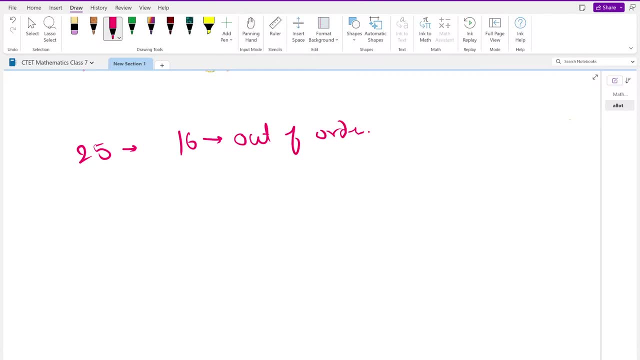 Out of Order. How many percent is bad? 16 Upon 25 X 100%, So 25 for the 100 And 16 for the 64%. 64%, 64%, Bad. Okay, I hope this time Everyone will definitely understand. No, No, Good. 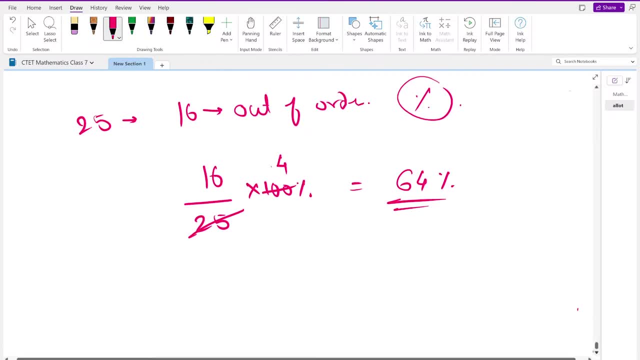 There is a shop. There is a shop In which there are 500 items. Okay, How many items are there in the shop? 500, Out of which 5 are bad, Out of which 5 are bad. So then, In the fraction 5 upon 500, X. 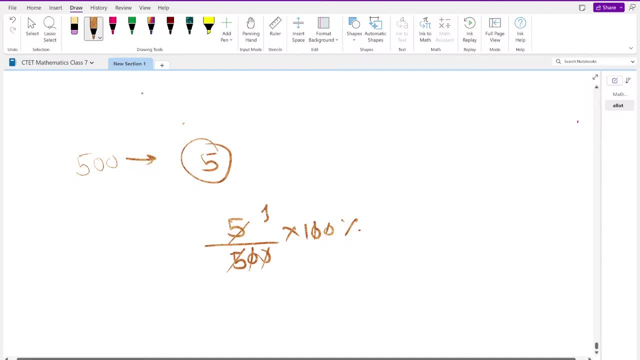 100% Cut Cut. Cut 5 by 5 Means 1%. 8 by 6, 6, 5, 7, 10, 8, 9, 11, 19, 20, 21, 22, 23, 24, 25, 25, 26, 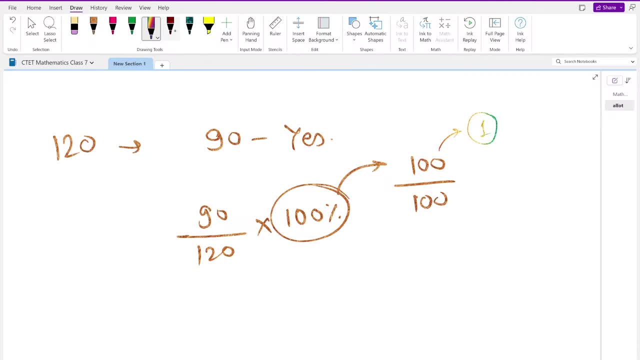 26, 37, 38, 39, 39, 40, 74, 74, 85, ilen 33, 34,, 3 by 4 into 100%, 4, 25, 25 into 3, 75,. so 75% people said yes and replied. I hope. 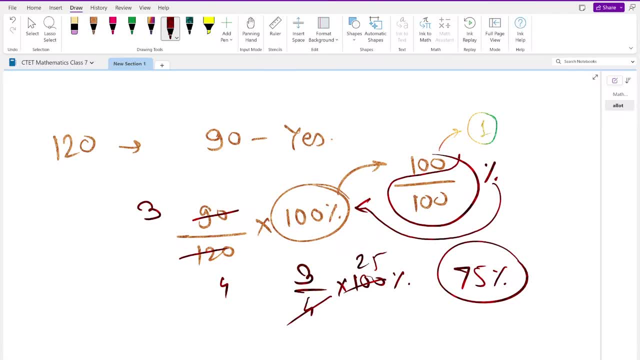 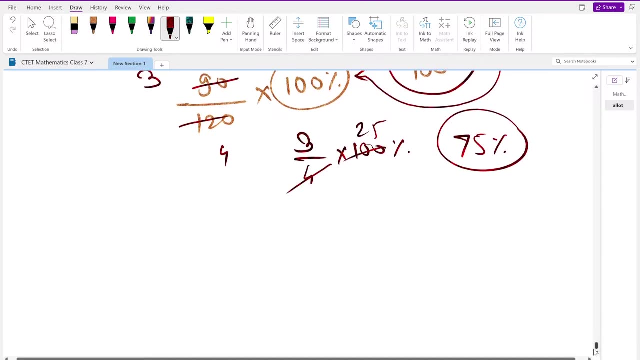 everyone understood this. okay, let's go. is there exercise after this? no, okay, lecture. how much time is left? 31 minutes? okay, let's go. let's increase the topic. okay, when you are teaching this in class, then for this at least give a week. this is a little difficult. 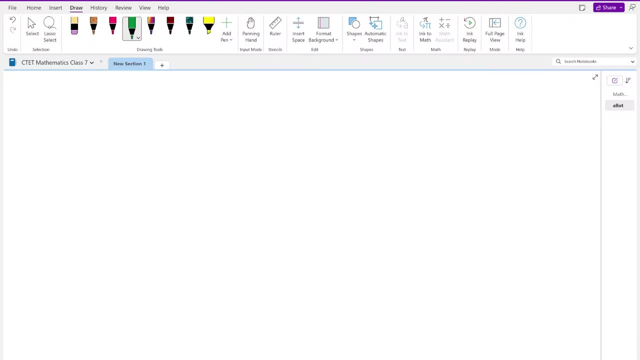 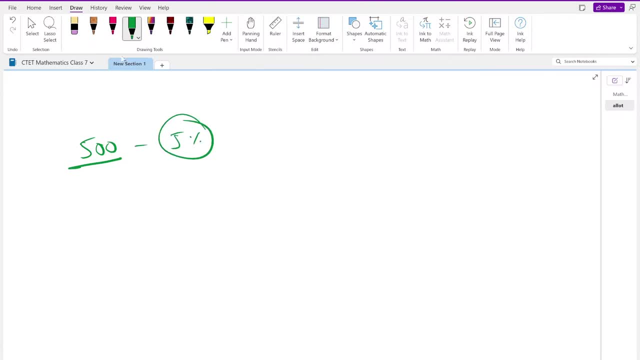 which 5% were bad. sorry, 5 were bad, ie one percent were bad. if 1 percent were bad, then 99 percent were good. 120 votes were there, out of which 99, if said yes, means 75 percent said yes. so 25 percent said not, said, said no. then you understand. 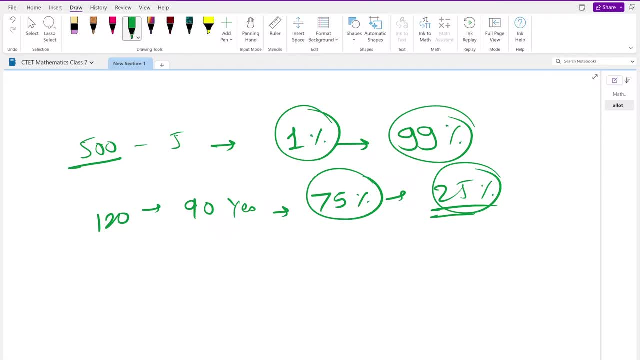 itself what it means to say that you can't tell me that yes or no, that your See if I write, there are 100% things, out of which 35% is of one type, so the remaining 65% will be of the remaining type. 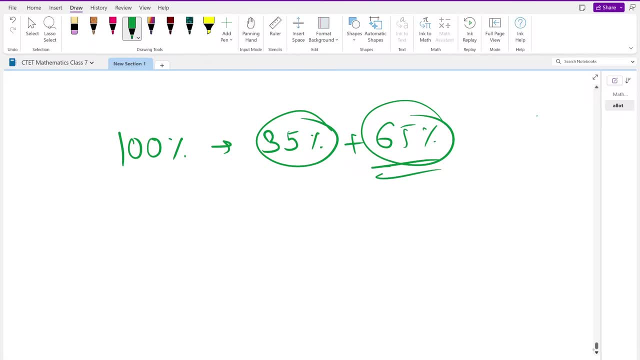 Do you understand this? Good, I write: one thing is 64%, the other thing is 20%. so how much will be the remaining thing? It will be 60%, so the total will be 100%: 64,, 20,, 88,, 4, 16%. 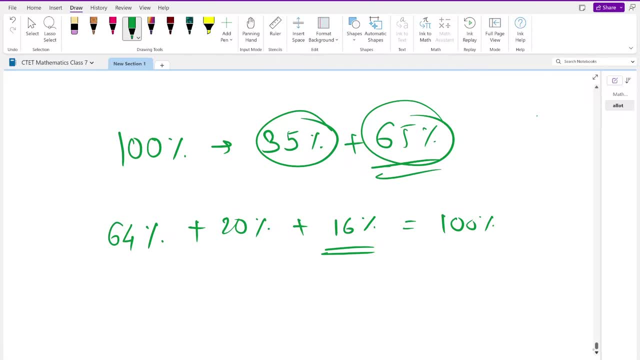 Sure, no one has any problem in this. It is just a part of subtraction. I hope no one has any problem in this. Now they have asked us a little question on the basis of diagram. For that we will see it in the book. 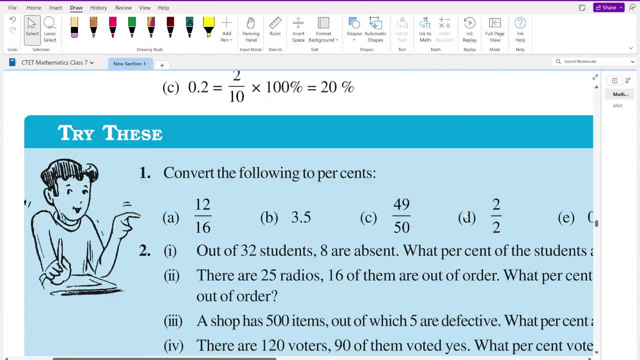 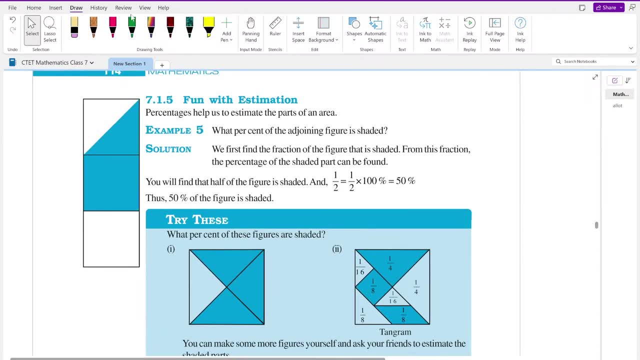 This is probably done. Now let's see here. He has asked us what percent of the adjoining figure is shaded. Now see, here we can see that half of the figure is shaded. So 1 by 2 means to convert it into a percentage. 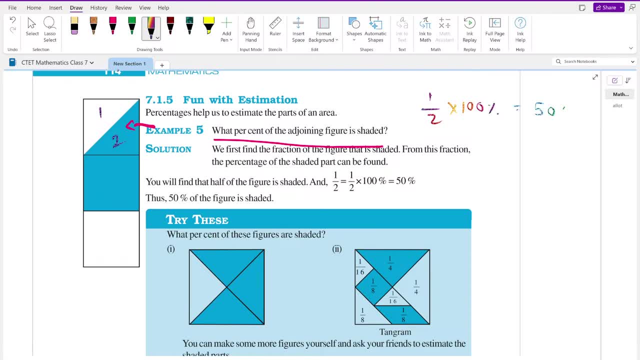 And 100 by 2 means 50.. 50%. So 1 by 2 fraction means 50%. Everyone will remember this. Okay, Now see here. There are 4 parts in total, 3 of which are colored. 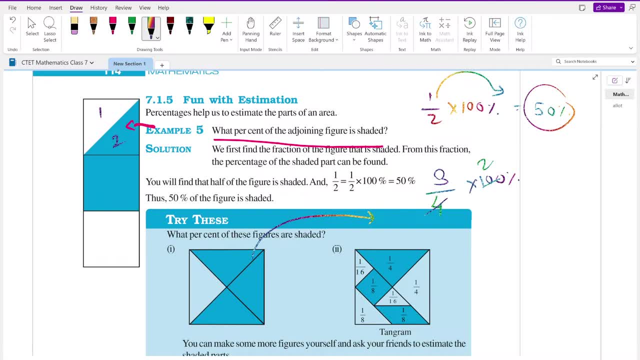 Into 100%. 25 means 75%. 3 by 4 means 75%. Always remember this. Okay. Now see, Shaded part is asked here. This is 1 by 4 plus 1 by 8, plus this is also 1 by 8.. 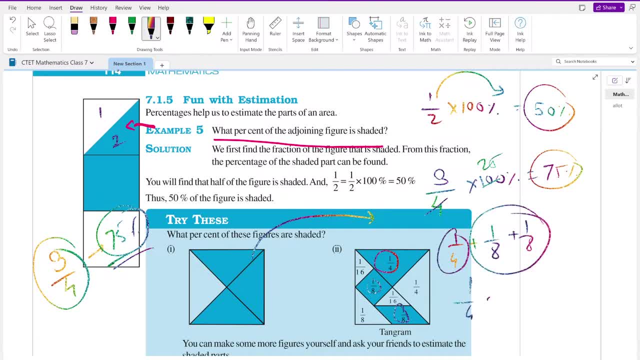 Leave this First. add these two: 1 by 4 plus 2 by 8 means 1 by 4 plus 1 by 4.. What happened 2 by 4.. What happened 1 by 2.. 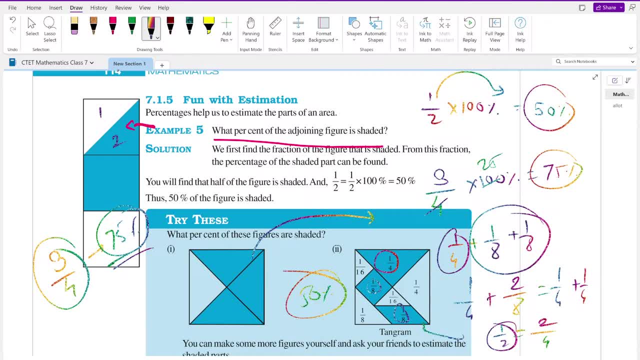 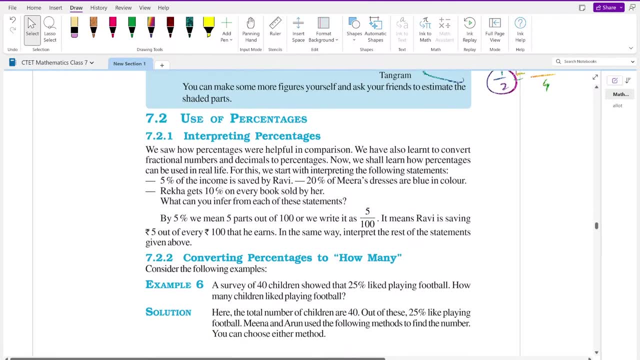 And 1 by 2 means 50% Understood. Very good, Okay, Come on. It is just an easy part. You should understand Now what is the use of percentage. We saw how we can compare with percentage. We can convert fractional numbers and decimals from percentage to percentage. 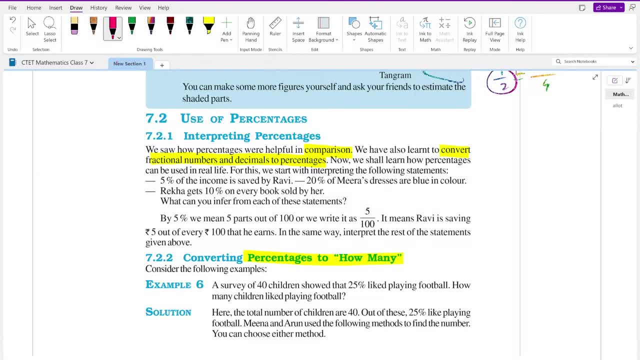 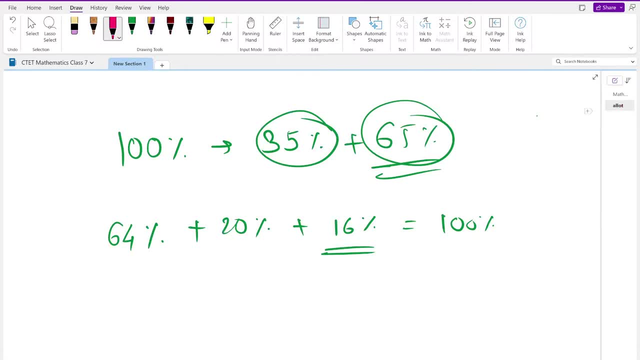 How can we convert percentage to how many? How? In a survey, 40 children. A survey of 40 children was taken. Okay, Let me explain the question. I mean statement: A survey was taken in which 40 students participated. 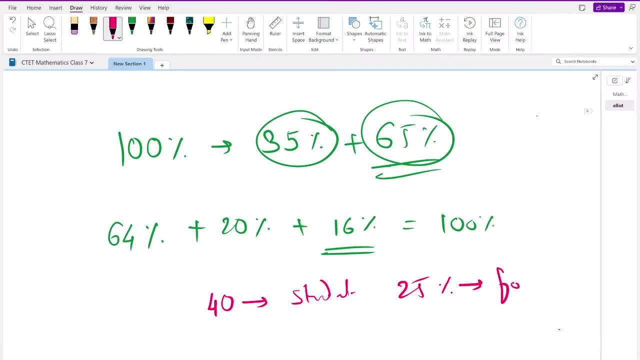 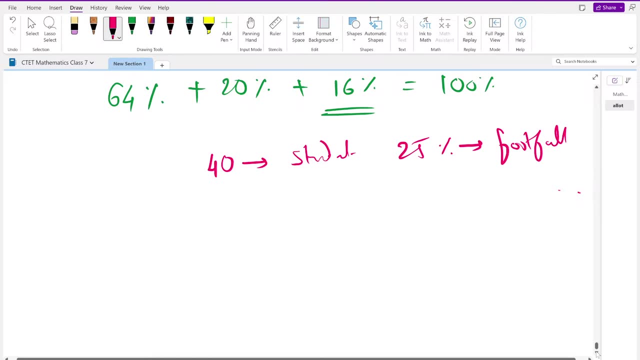 In which it was said that 25% of students like football. 25% of students like football. So how many children like football? We were asked this question. Okay, Come on Now. how do we solve this? Let me show you. 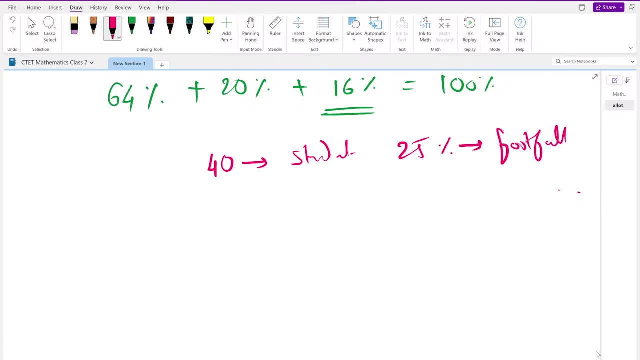 Let me show you Now, see, There are two ways to solve this. Out of 100 children, 25 children like football. So out of 40 children, how many children will like football? And by doing its cross multiplication: 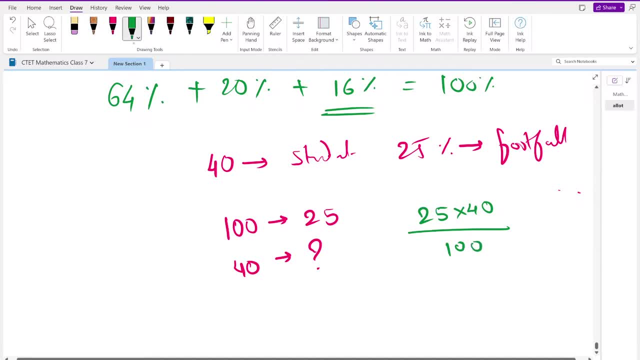 we can solve 25 into 40 upon 100. Okay, 25 ones are 25.. 25 fours are 4.. 10s are 10 students Out of 40, 10 children like football. Okay, This is an easy way to solve the problem. 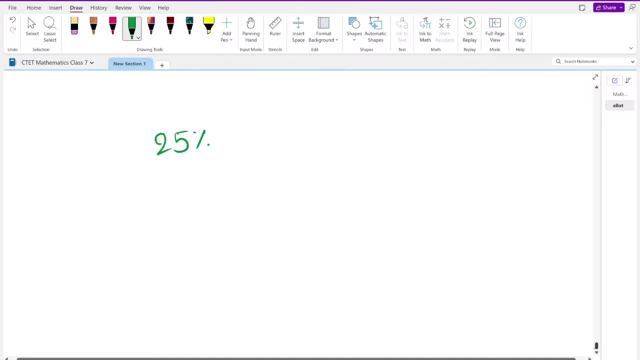 Or 25% to children, 25%, which Of 40. Right, How will we get 25% out? 25% of 40.. 25% x 40 and % means 100, 25 x 100 x 40. 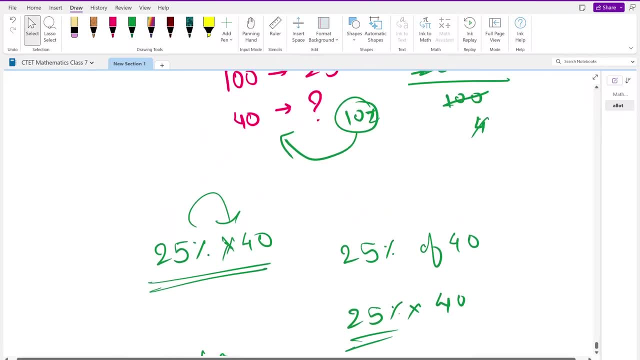 see here. what will we say? the same equation came up: 25 x 40 x 100. ok, it will be same. you just have to solve it according to your own way. got it ok? now we are asked a question: 50% of 164. how will we solve it? 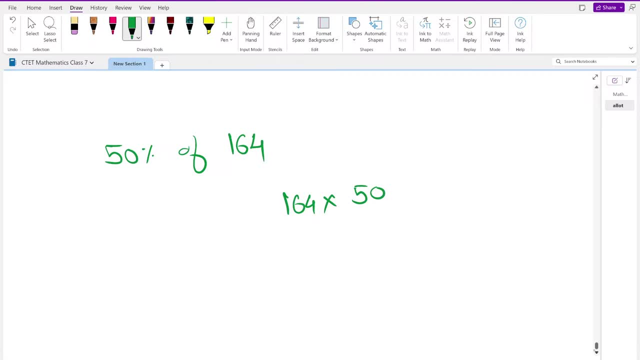 after saying off. there is a multiplication sign. 50% is not this: 50 x 100, 0, 0, 1 x 2. 164 x 1 x 2. 50% comes in your mind after seeing it. you have to do half of it. 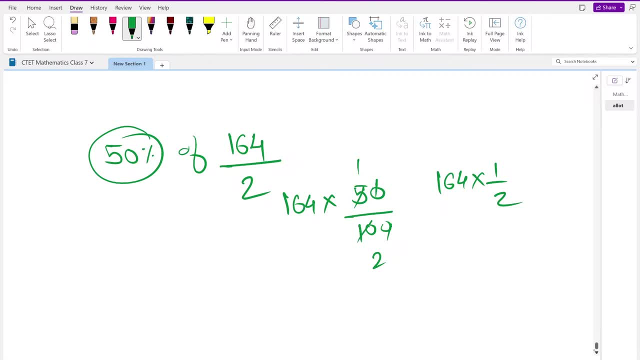 ok means when you are studying as a teacher, you will know this. 2 x 8 is 2 x 2 is 82- 82 got it ok? come on now we have to talk about 75% of 12. after saying 75%, you also have to remember 3 x 4. 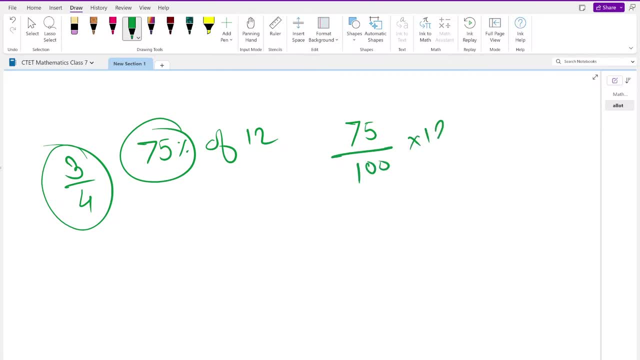 ok, how: 75 x 100 x 12 and from 25 table: 25 x 3 is 25 x 4 is 3 x 4 is 12, 4 x 3 is 12 means 9, 25% of 12 is. 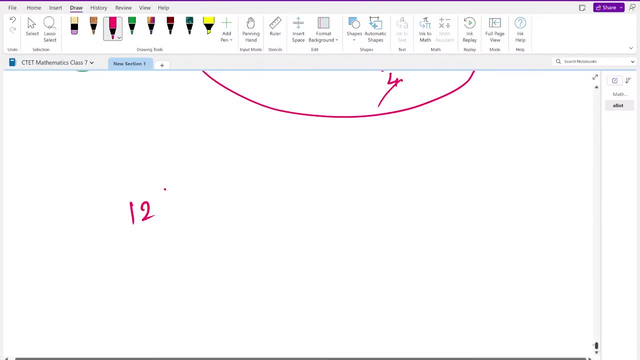 9. can anyone understand for sure? ok, 12, 1 x 2 % of 64. how will we solve this? first in fraction. convert it in improper fraction, and that is 25 by 2 into 100, into 64. from where is this into 100? 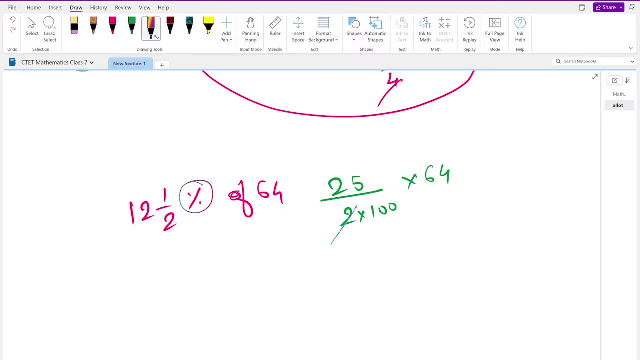 this is in place of percentage. ok, let's solve it. 2 x 3 is 2 x 2 is 25 into 32 upon 100. 25 x 2 is 50, carry 5. 25 x 3 is 75, 75. 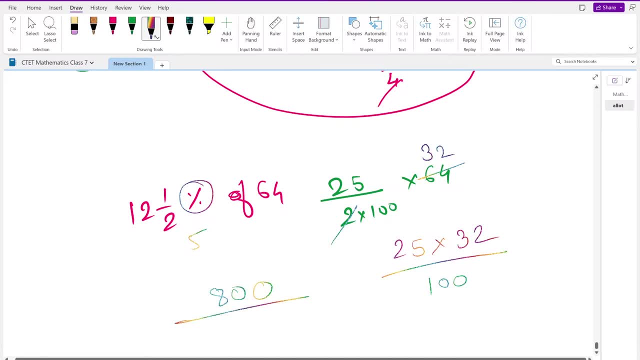 75 plus 5, 80, 800, 9 x 2 is 50, 9 x 3 is 75, 80, 9 x 3 is 7, 6, 8, 10, 10, 11, 11, 12, 14. 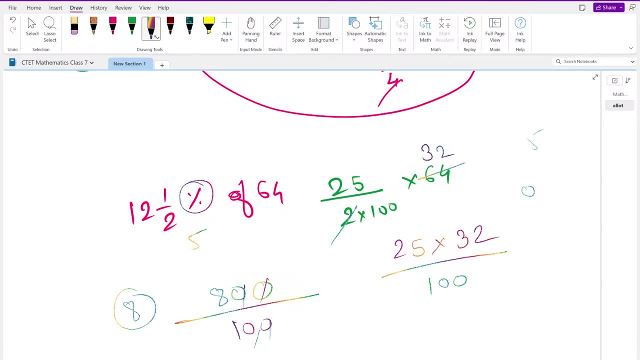 15, 18, 17, 28, 29, 30, 22, 24, 25, 26, 27, 28, 29, 30, 31, 32, 34, 34, 35, 36, And because of this I have solved these questions only. 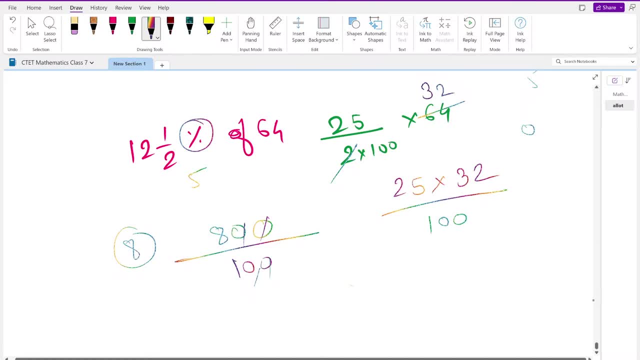 Okay, this final answer was 8,. I have written it In the next lecture. oh no, two questions are remaining. In the next lecture we will start the actual exercise, And if you watch this lecture well, trust me you will benefit a lot from the rest of the competitive exam. 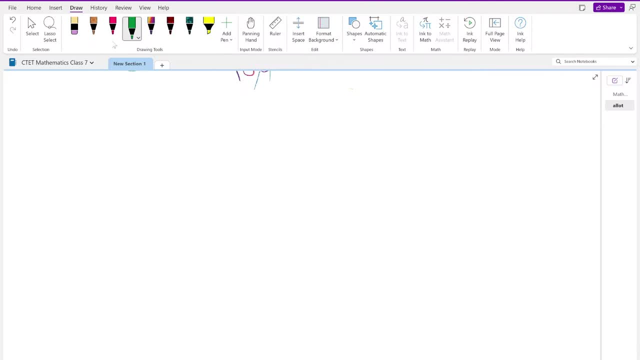 Okay, this is really really helpful. Okay, last two questions: 8% children of class 25 like getting wet in rain. 8% of the students like getting wet in rain. 25% of the students like getting wet in rain. 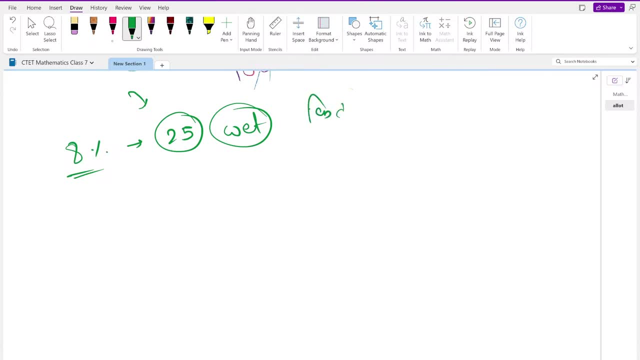 So how many students like getting wet in rain? Now see, we can solve this in two ways. First of all, 8% of the students like getting wet in rain. So how many students like getting wet in rain out of 25 students? 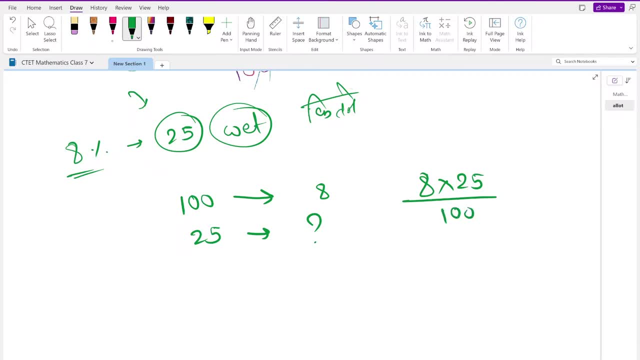 So cross multiplication 8 into 25 upon 100. This is one way. Second way: 8% of 25 means 8 by 100 into 25. And that will be equal to see, both are same equations. 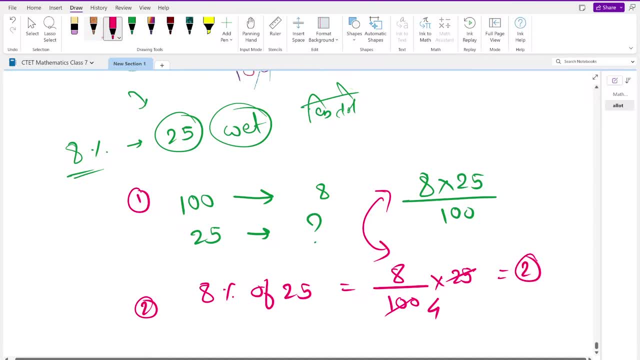 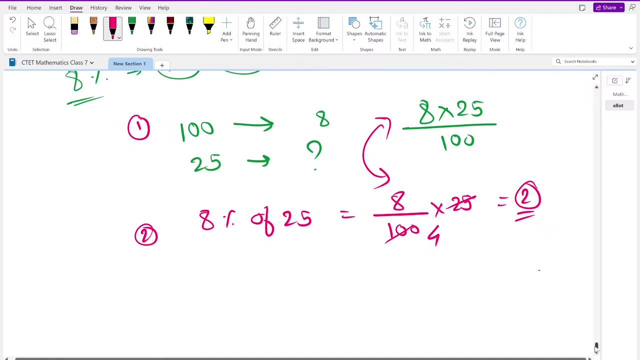 25 for the 4 to the Means. out of 25, how many students like getting wet in rain? 2.. Out of 25, how many students like getting wet in rain 2.. I hope everyone understood this. 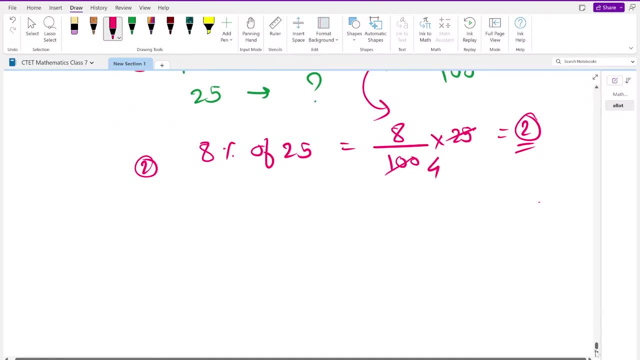 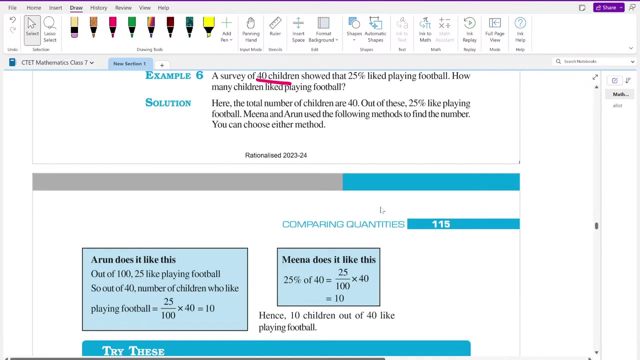 Okay, moving on to the last question of our not exercise. oh no, there are two more questions. Okay, no problem. no problem, Rahul bought a sweater. I am telling you this question in the book. Okay, I told you that you should have the book. 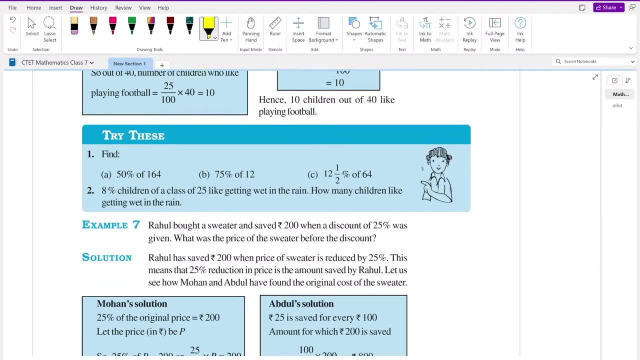 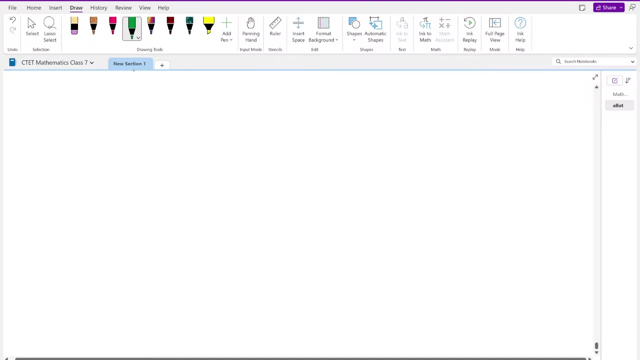 Okay, I am telling you this question. Rahul bought a sweater and saved Rs 200 when a discount of 25% was given. Okay, let me tell you, He got a 25% discount on Rs 100.. Okay, so he got the benefit of Rs 200. 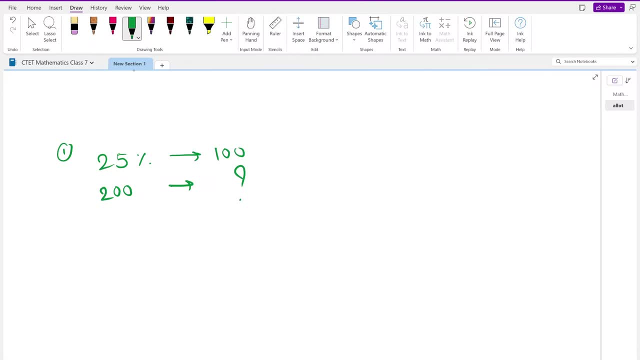 So what is the actual amount? We were asked this question. Did everyone understand this? What did I say? Rs 25, percentage. sorry, I wrote it by mistake. I got a discount of Rs 25 if that thing was of Rs 100.. 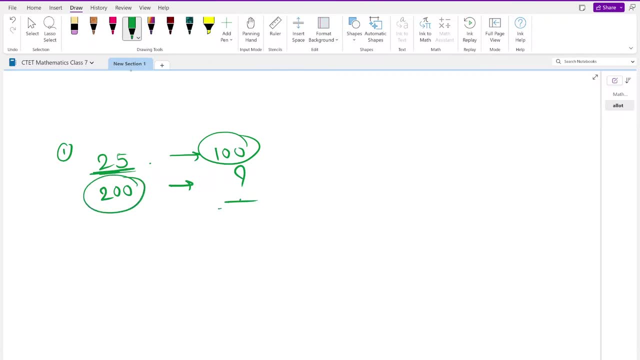 But we got a discount of Rs 200 in actual. So we were asked: what is the value of that thing? So we will cross-multiply it 100 into 200 upon 25.. This is one way. Now I am telling you the second way. 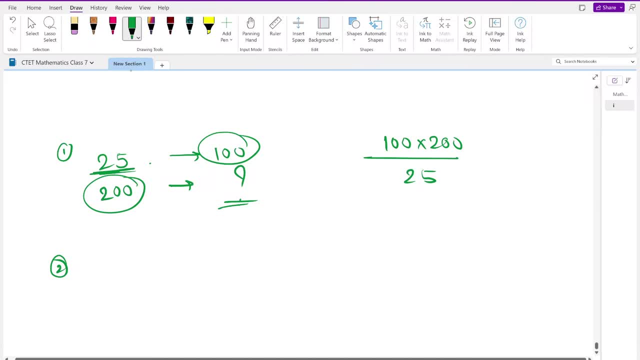 Everyone will pay attention to this. Now assume what is the value of 25% of any thing: 200.. Then what is the value of x, 200 upon 25%, Which is 200 into 100 upon 25.. See, both the equations are the same. 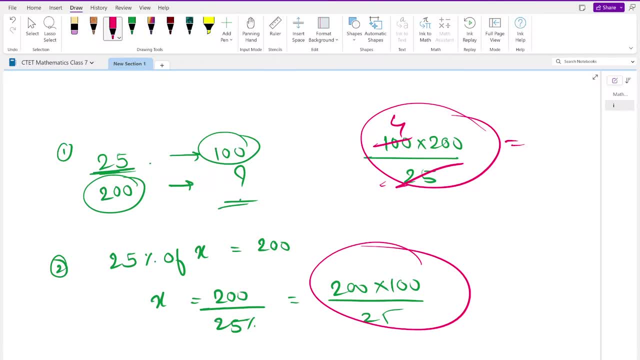 Okay, it is also easy to solve this: 25 for the 800.. Okay, what is the value of that thing? 800.. Here also 800.. Which method are you using? This does not matter, Because both have the same answer. 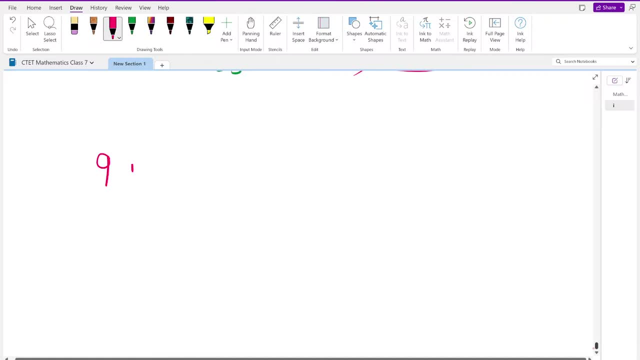 Okay, Come on, pay attention. 9 is 25% of a number. Now see, we can solve this in two ways. First, we know a number. If we don't know, then we assume x, 25% of x, is 9.. 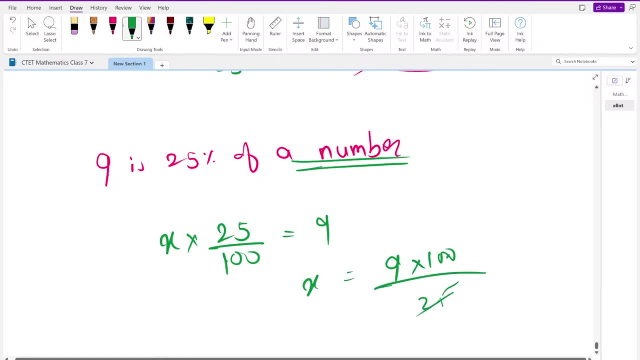 x is equal to 9 times 100 upon 25.. 25 for the 9 for the 36. So that number is 36.. This is one way, Or then that number is 9.. 9 out of 100.. 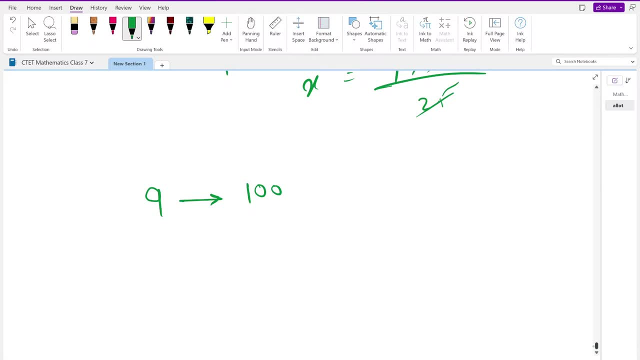 So then, what is that number? now, Okay, I will tell you what happened. When we assume that number as 100, then that number is 25.. But actually that number is 9.. So when 9 is that number, 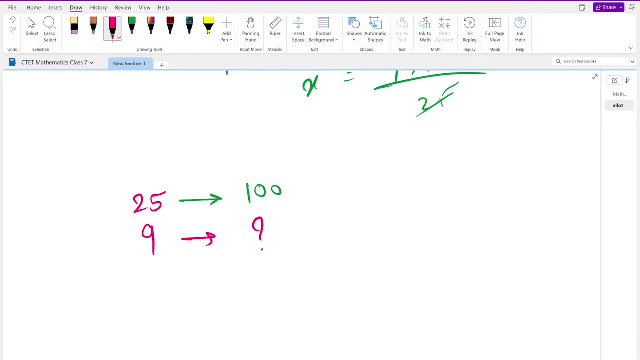 then what is its value? What is its original value? So this is the crock multiplication 100 into 9 upon 25.. Done, Okay. Now see it is saying that 75% of a number. When I say a number, 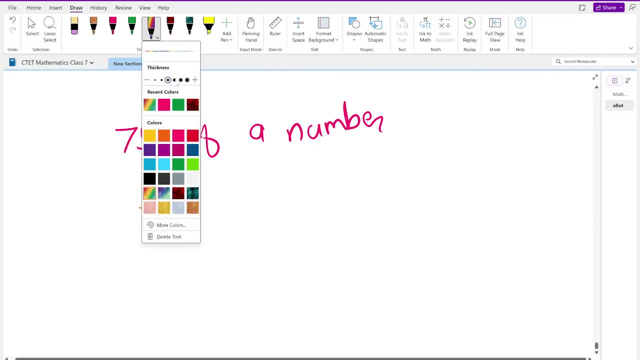 I mean x, 75 upon 100.. Into x is equal to 15.. It is given in the book. So x is equal to 15 into 100 upon 75.. 15 times 5 is 75.. 5 times 2 is 1000.. 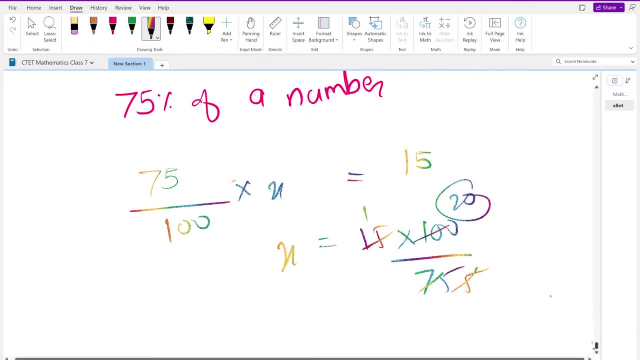 So then, what is that number? 20.. So x is equal to 20.. Now in the exercise 7.1, there are approximately 10 questions And all its questions are 25 to 30 questions. Okay, So. 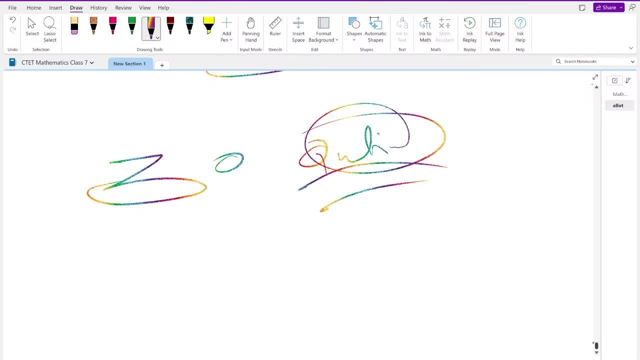 in our next lecture we will solve those 30 questions. Okay, I hope no one has any problem till now. Everyone must have understood. If not, then send a message. You have that option here, Okay, Okay, Bye-bye and take care. See you tomorrow.